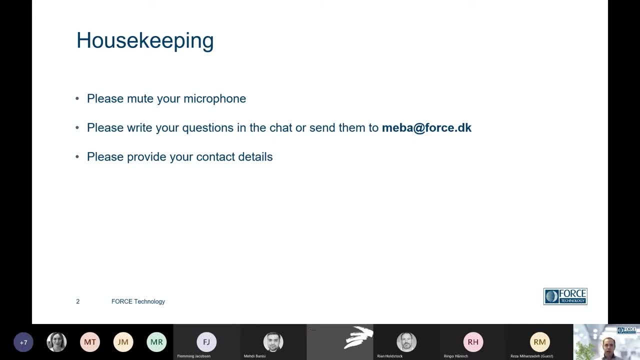 feel free to write them in the chat. We're going to have a break after the first presentation and then after the second for questions. Now, if your question is something that you don't want to share to the large forum, you can. You can write the question to my colleague, Mehdi. His email is here: meba at forcedk. 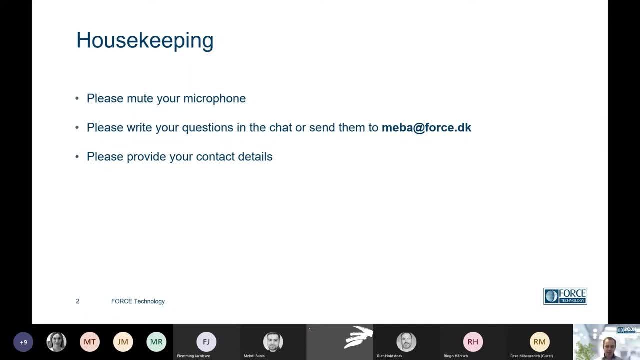 or really get in touch with any of the FORCE people And please provide your name and contact details that if we don't get to all the questions during the session, that we can follow up with you after, because we don't want to leave any questions open. 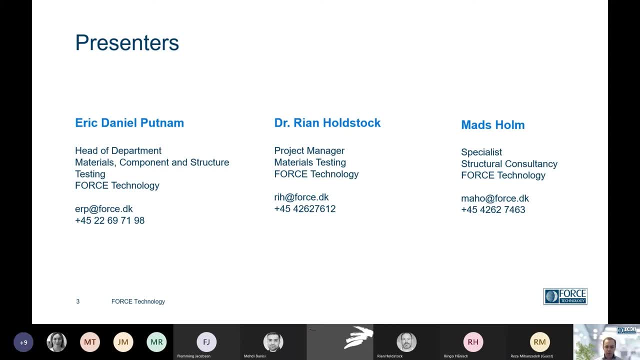 So just to you know, move along. there are three people from FORCE here today. Myself. my name is Eric Putnam. I'm head of department for the materials, component and structure testing teams. We have Rian Holtstock. He's a project manager within materials testing. 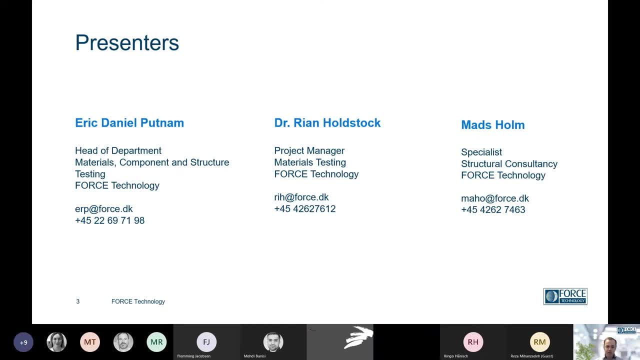 Rian will be giving the first part on kind of the background and basics within fracture mechanics testing, And then we have Mass Holm who's a specialist within our engineering consultancy area, And Mass will be giving going a little bit more on the engineering. 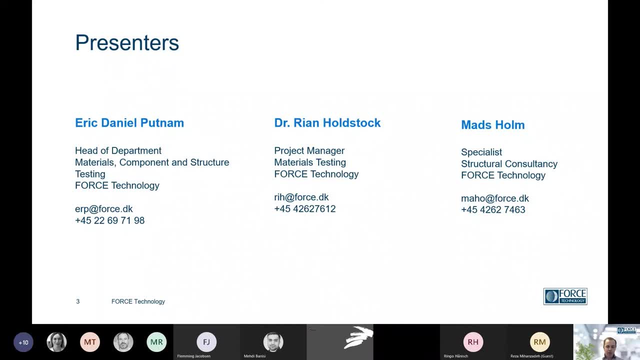 critical assessment and the link into the testing programs. So that is the end of the session, Thank you, Thank you. So that is the end of my part And I will now pass off to Rian who will go into fracture mechanics testing. 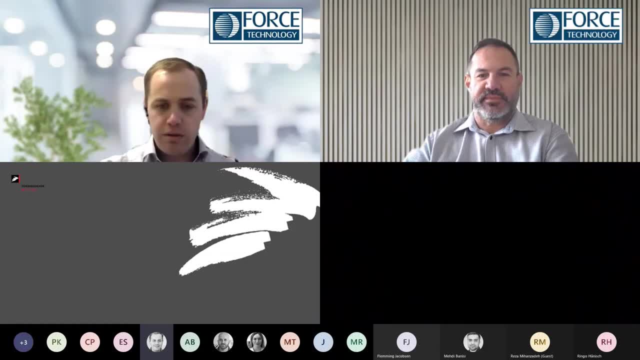 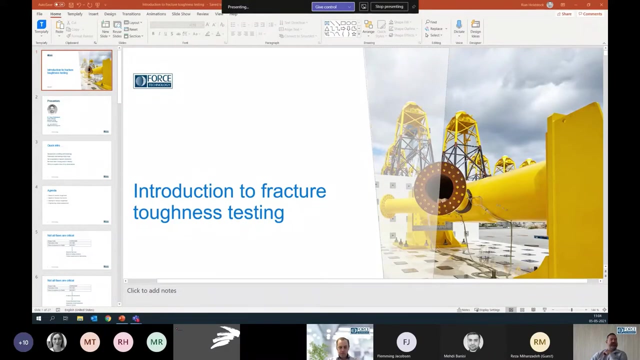 So, Rian, I'll stop sharing And you're muted, Rian, There we go. Thanks, Eric. Right, Let me just share my screen here. There you go, Okay. So, Eric, can you see my presentation? We're good to go, Rian. 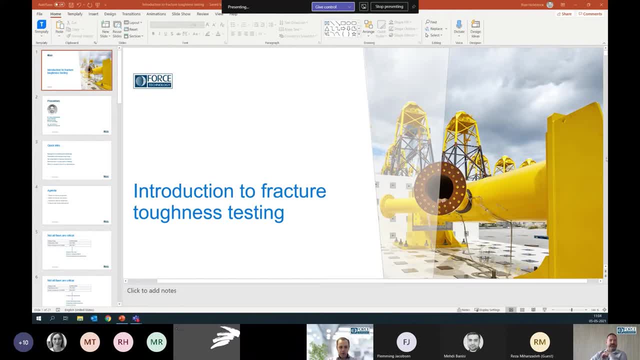 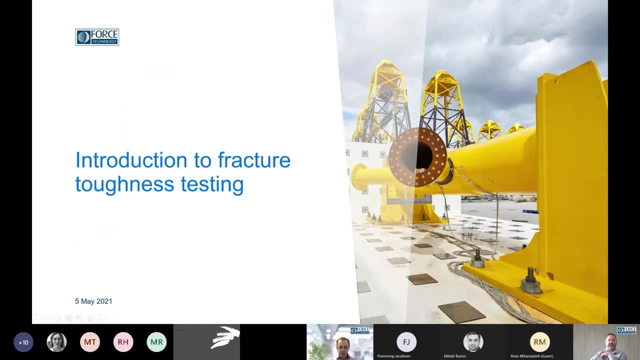 Okay, So they just need to make it full screen. Yeah, there you go. It should start now. Does that work? We're all set Beautiful, Okay, Well, welcome to today, And thanks for the introduction, Eric. Thank you. 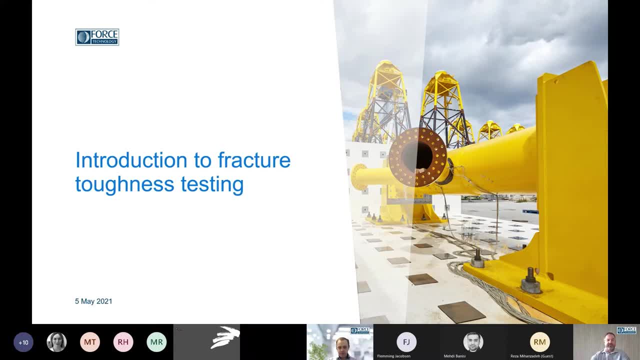 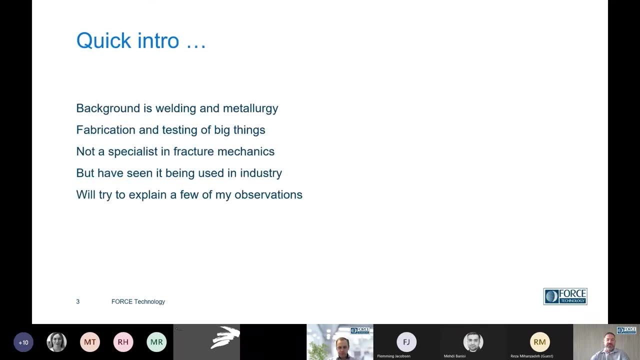 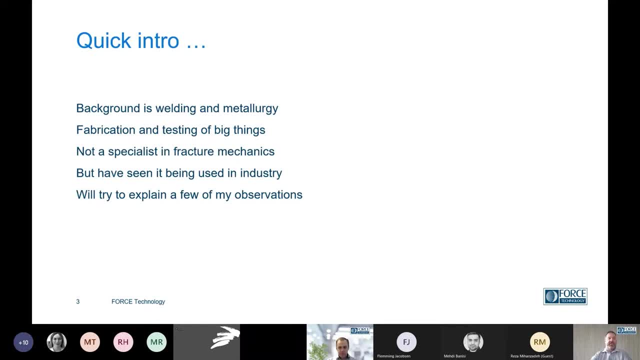 not a specialist in fracture mechanics in any way, but I've seen it being used in industry and I'm involved with it now and again. But it's pretty much like a car. You know how to drive a car, but you don't know how the thing works. You just know: get in, put the 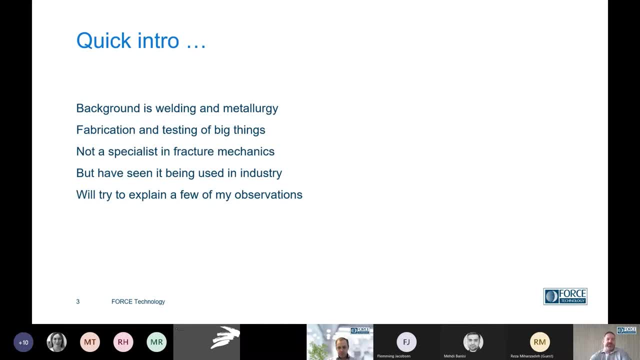 key and turn the ignition off, you go, And that's pretty much the same as me. But what I will try and do is explain a few of the things that I've seen, And my big aim is to build a bit of background for what follows next afterwards with the next presenter, when 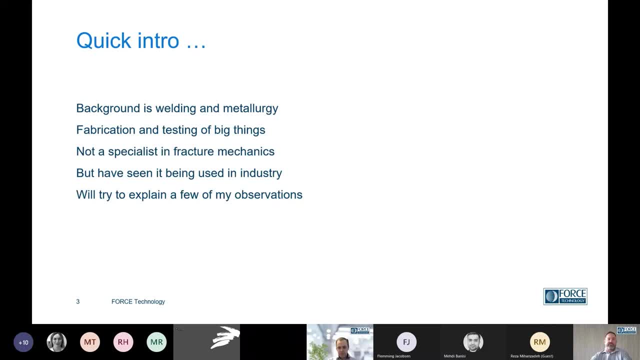 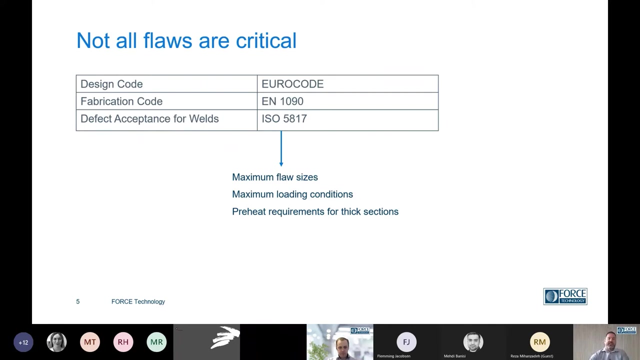 Mads will tell you: Okay, The other things Right. So the agenda is: basics, Basics of fracture mechanics, basics of fracture toughness- How do we test for fracture toughness? And also- I'll just introduce this engineering critical assessment. Now, before we build something, we need to go through. 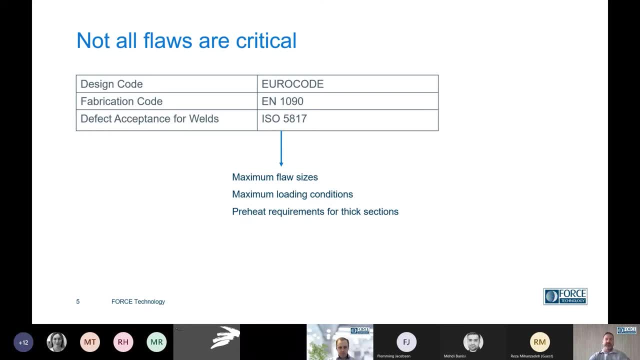 paperwork, and I'm sure most of you probably already know this. So the example we can see. there Are some specific rules that tell us about the flaws in the structure And one important thing is that it talks about a maximum floor size. Now, these things are mostly conservative. 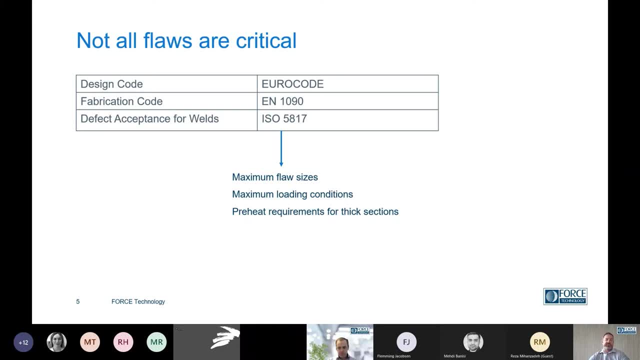 And, as we know about conservative things, it makes things more expensive and it also slows down the work. Oh, Okay, Okay, Okay, Thank you. Then we ask the question now: is there an alternative? Is there a safe alternative? What can we do? And that is the theme of today. So I will introduce the basics and then, hopefully, 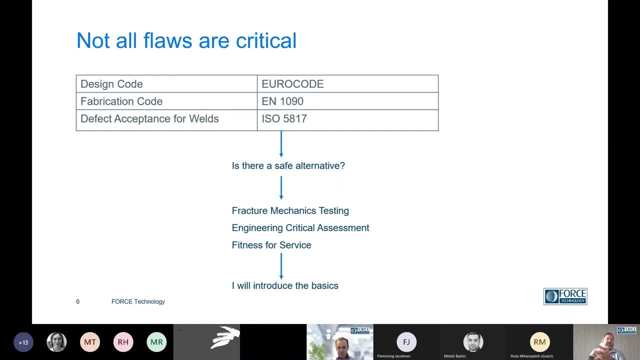 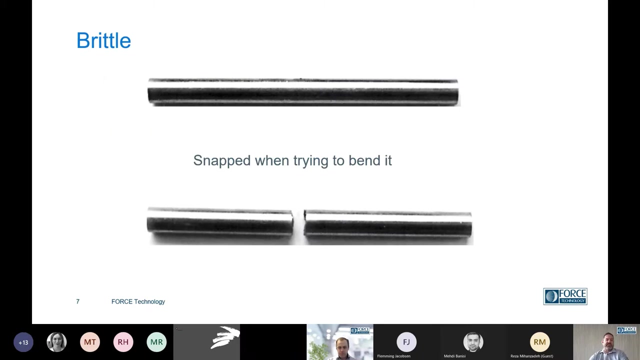 that, if you don't already have it, it'll give you a little bit of an understanding of how we can go about using a safe alternative rather than using the Yes, using the conservative approach given by the codes and standards. OK, so in case there are some of you who are very new to this, 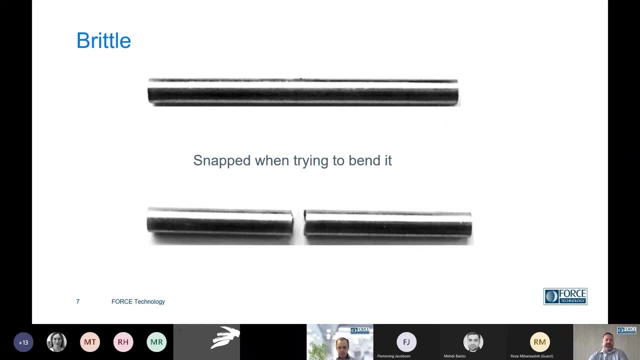 I'll start very basic and I'll ramp up a little bit. So let's introduce the word brittle. And what does it mean? Very basically, where easily it takes something and you bend it, or you try to bend it and if it snaps it's brittle. 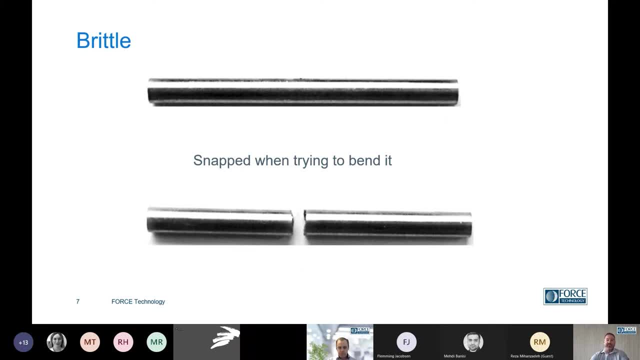 The important thing is there was no deformation. Then, if we look at ductile, we see the opposite: There is deformation and it did not snap during bending. So this deformation, that's the word that I'm starting with. If there's deformation, this is going to take us into the fracture mechanics part. 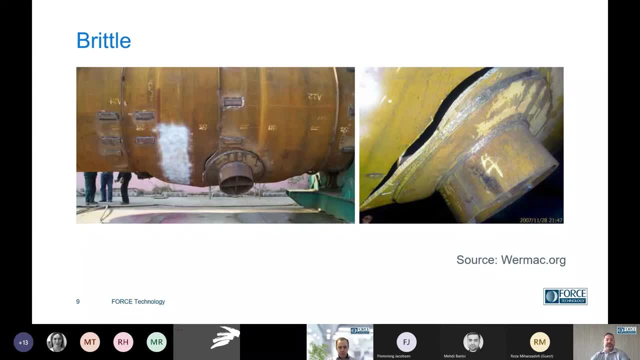 Now here is an industry example of a brittle fracture and we can see that around where the fracture was There was no deformation. So that is a very easy way to see that this was a brittle fracture. If we go to a ductile fracture, we see this pipe here. 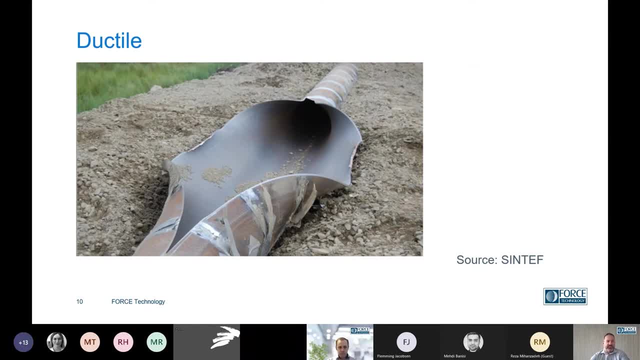 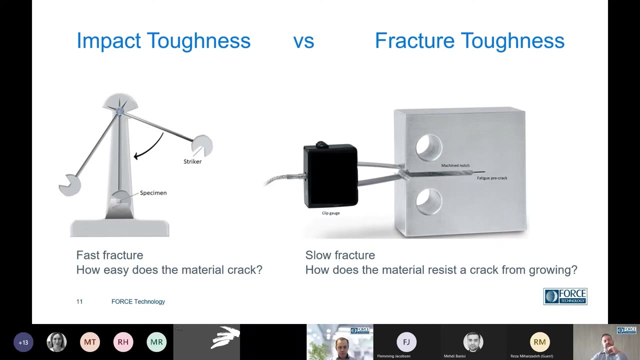 There is deformation and so very easily we can see one was a brittle fracture and the other one was ductile. Okay, so that was easy. but now I also have to separate impact toughness from fracture toughness, and they are not the same thing. 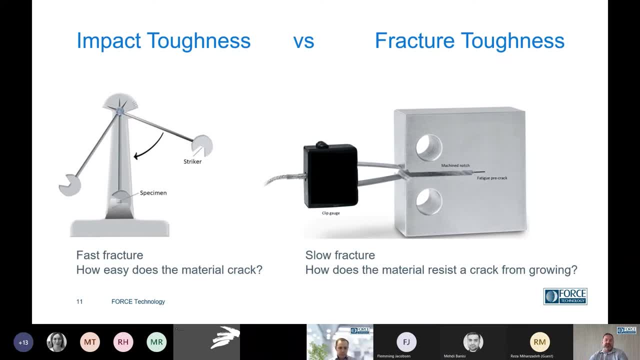 Impact toughness gives us a fast fracture and gives us a quick general assessment, But if we want to evaluate a material's fracture toughness, we need to go a bit more deeper. We need a A lot more work, and the example here shows a typical setup for fracture toughness. 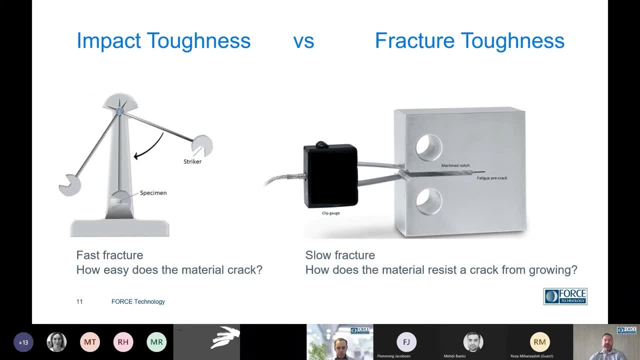 If we look on the right hand side, the specimen will be pulled apart. We throw in some mathematics, close control of the loading conditions, the specimen geometry and that little black thing there that measures how the crack grows or not. the crack grows, but it measures how. 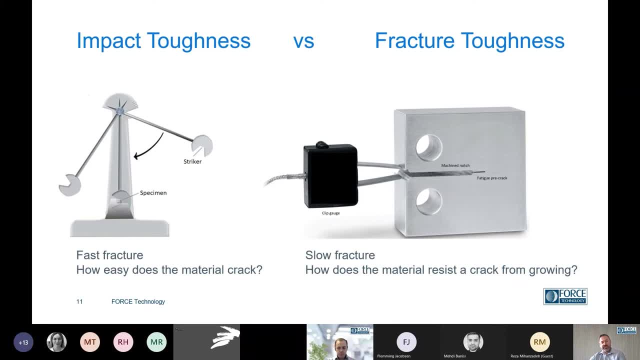 the front of the crack or the face of the crack is opening up And we do some analysis after the specimen has fractured And very simply that gives us a basic description of fracture toughness. So of course, impact toughness on the left is just put something. 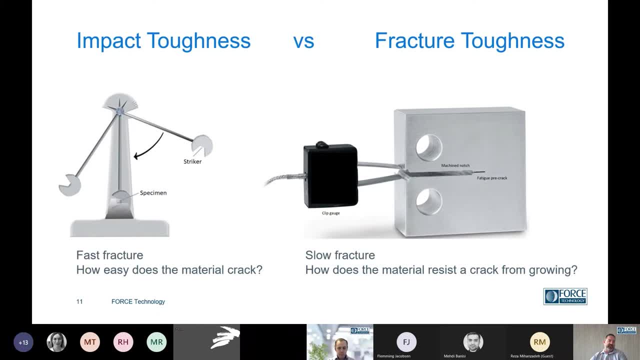 put the specimen in there, release the striker very quickly. it fractures the specimen. That gives us the impact toughness, Whereas the fracture toughness on the left is just the impact toughness. We need to look at what's happening more closely at the crack tip. 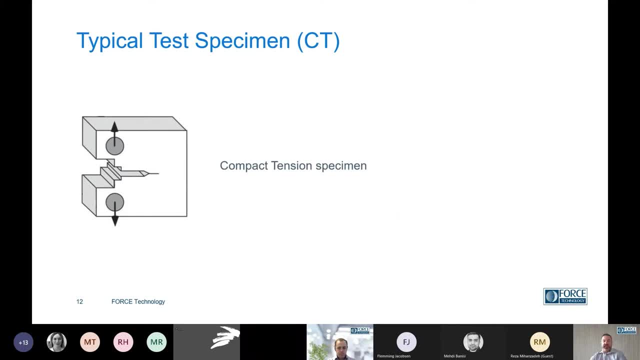 OK, a typical test specimen. here we see a compact tension specimen. Now, as the word says, it's tested in tension. The specimen geometry is important, So things like width, height, length, these have to be closely controlled. We also see that there's a machined notch. 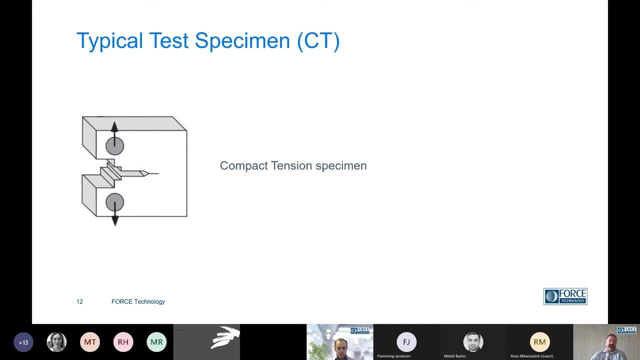 And sometimes there's a fatigue pre-crack. So here's our machine. Hi guys, Just mute your microphone there, please, Unless you have something really important to tell me, if I can just ask you to mute your microphone. So if you look at that drawing there on the left-hand side, 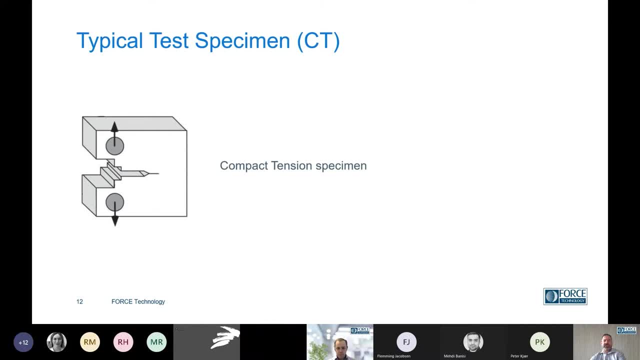 there's a machined notch and then there's a small straight black line. Sometimes there's a fatigue pre-crack put in there And what that does. it helps us to have a very accurate starting condition for the test. Next one to consider is a single-edge notch bend specimen or SENB. 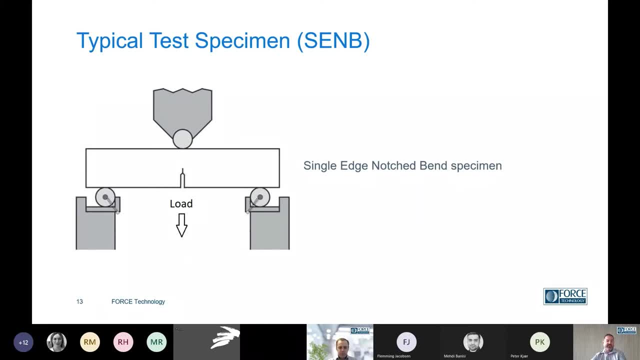 It's bigger than the previous one, the CT specimen, And the other one was in tension. This one is in bending But, just like before, the geometry and the starting conditions are very important. The final specimen that I want to introduce, which, of course, these are not all the specimens. 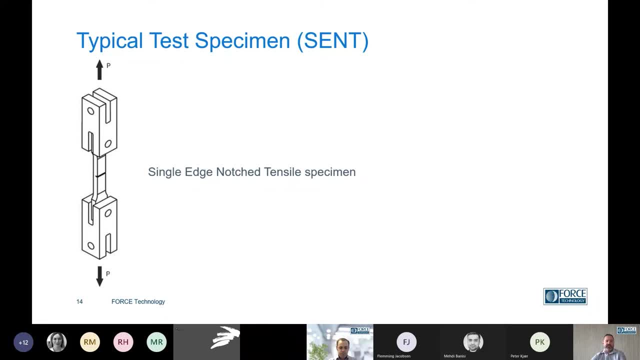 it's just the three, four. today that I want to introduce to you is a single-edge notch tensile specimen. So it's a tensile test, but with a notch, and it's also relatively thin. and remember there that the geometry is important when 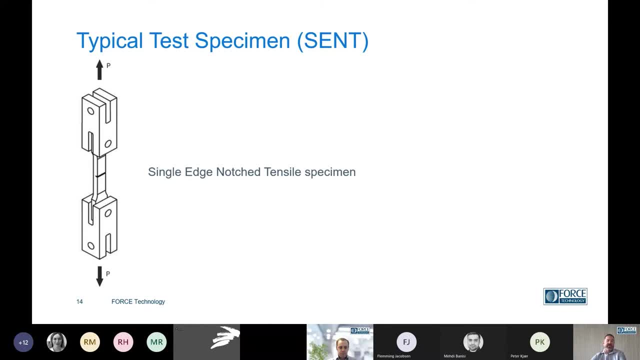 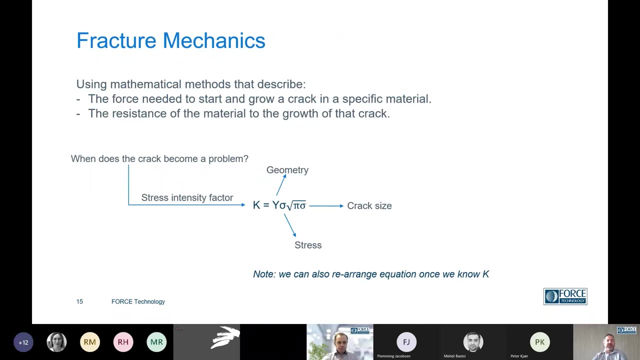 we have to decide or when we have to design a fracture toughness test. So I'm throwing in words like geometry, because we'll see later where this comes from. Okay, now let's have a quick look at fracture mechanics. Now, these are my words. as I said, I'm not a specialist. I'm just giving you my understanding. 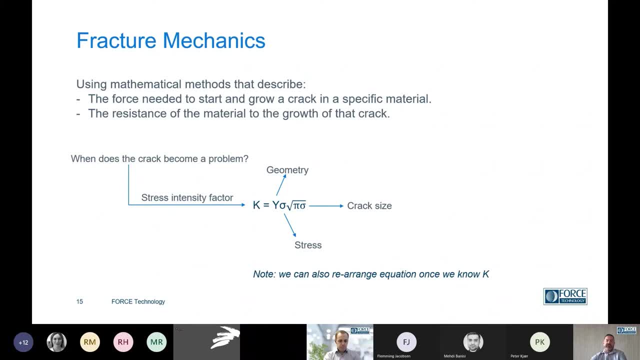 of it. So fracture mechanics uses mathematical methods to describe the force needed to start a crack and also the resistance of the material to the growth of that crack. So when does a crack become a problem? This example here. if we look at that in the middle, there it's a crack that 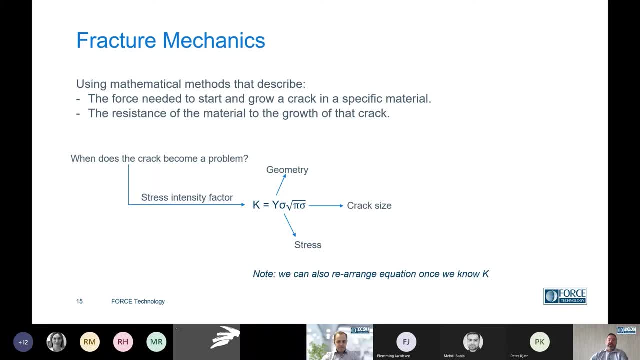 there's something called a stress intensity factor and it's a k, and if we look a little bit to the right, to the equal side, we see that geometry, crack size and stress, these are important things. So if we look at the crack size, we can see that it's right next to the geometry. 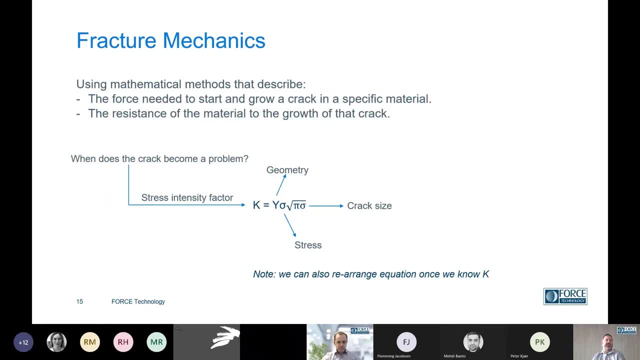 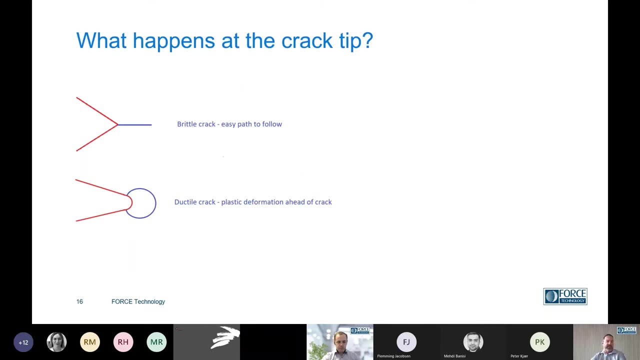 So this is a clear link between the geometry of what we test and also how the crack behaves. And to be able to illustrate this a little bit better, we will zoom in a bit and we see what happens at the crack tip. So very, uh, simplistically drawn there, we see that we got a brittle crack and a ductile crack. 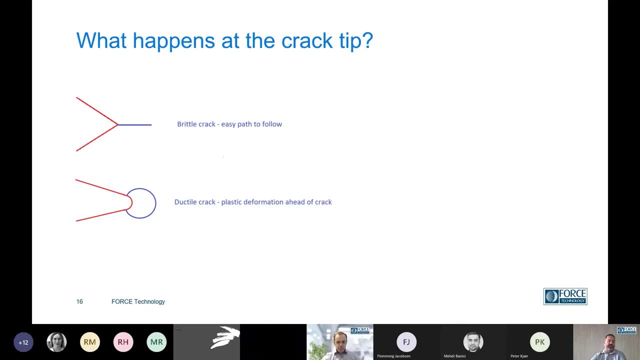 Now the red is the crack and and that blue line or the blue circle that represents the area in front of the crack. So a brittle crack? um, it's a straight line? there's not. it's very fast that if the energy needed to propagate the crack, to make the crack grow is is not a lot, whereas 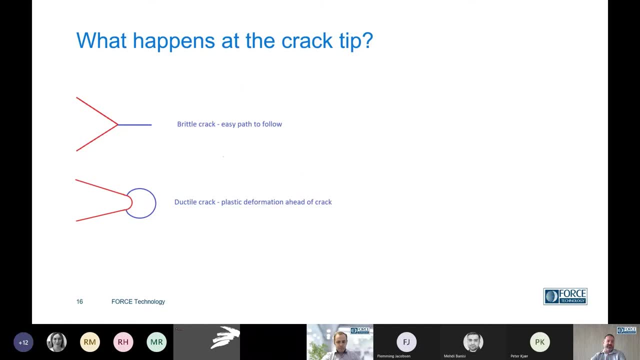 if we look at a ductile crack, we we see this circle in front and- and that tells us that the crack doesn't have a straight path- There are some other things in there that is stopping this crack from from growing, and the more work is required to make that crack grow, 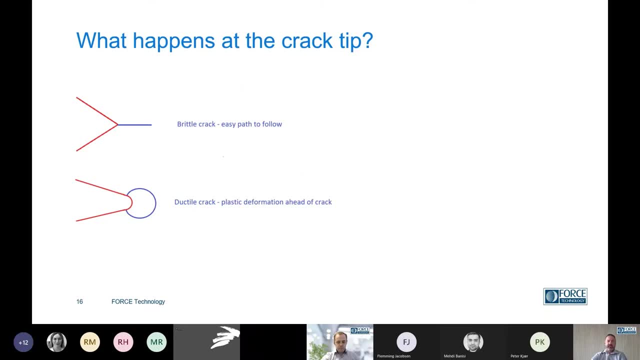 the higher the fracture toughness will be Right now. another important concept here is is the. the slide shows three examples of how the plastic zone can behave. um, because it tells us whether we're looking at linear or non-linear. The most common one is that the black line is straight and the red line is one and the 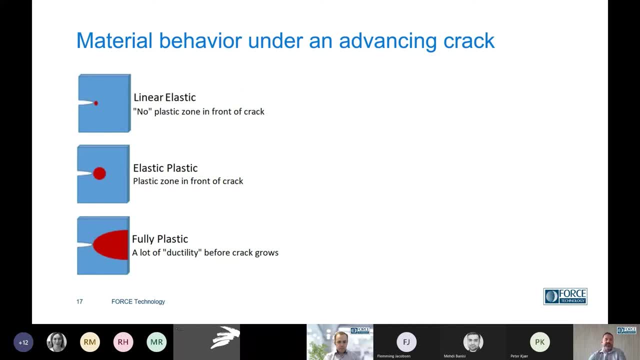 black line is two, so it's a combination of both. of course, the black line is straight and the blue line is non-linear, which is the most important differences. The black line is straight and the blue line is one plays an important role here, and this is why We've got something called plain stress versus 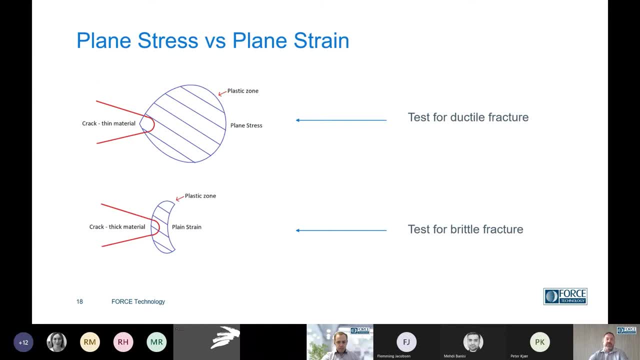 plain strain and these conditions affect what happens at the crack tip. So under plain stress conditions we have a large plastic zone so a lot more energy is required to make this crack grow and we'll find that thin materials will generally give us a plain stress condition. 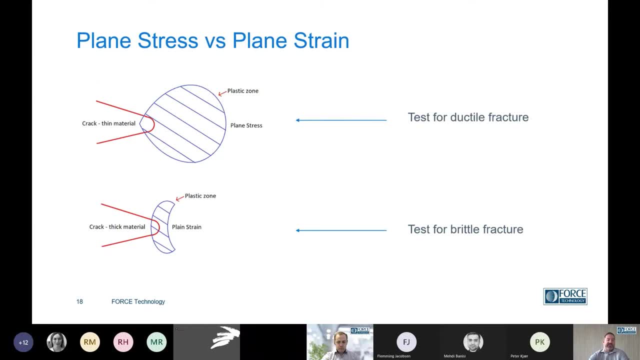 whereas if we look at a plain strain condition, the plastic zone is smaller and this is typically what we will see in thicker materials. So, to generalize, if we want to test for ductile fracture, we can use thinner materials. but if we want 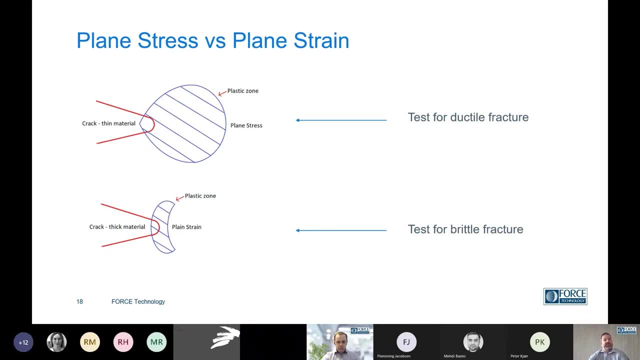 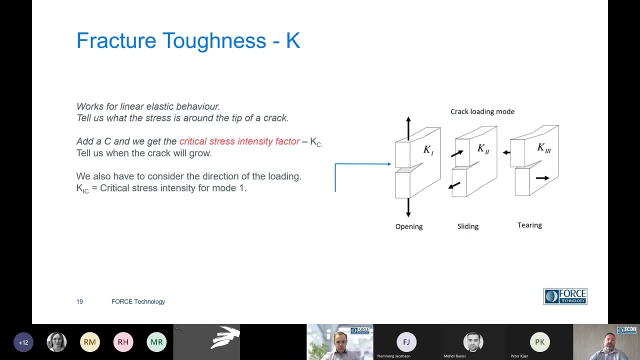 to test�� for a brittle fracture, then we need to go to thicker materials or a thicker test specimen. all right, go back to to this fracture. toughness again, this stress intensity factor. so if we add a c to it, kc, then then we get something called the critical stress intensity factor, and so not. 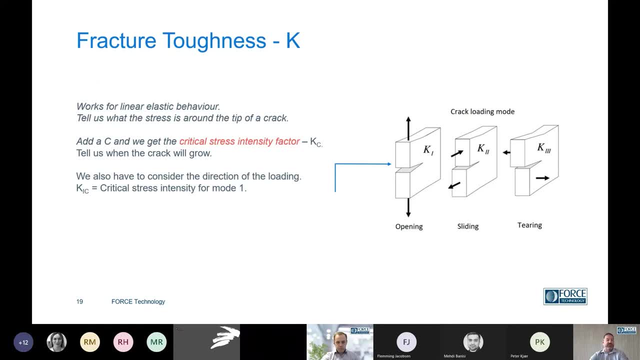 just do. we know what the stress is at the crack tip, but we can also find out what stress is needed to make that crack grow, and that becomes the critical part of it. and then, as, as we can see, there's a one, two and three there. that gives us, uh, the different ways of offer. you know the different. 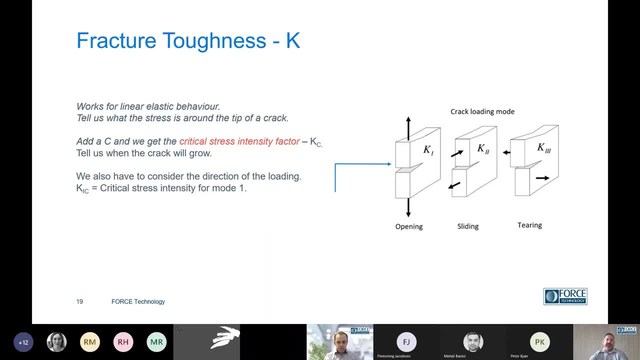 modes of the fracture. so k is our first way to describe fracture toughness. it's our first parameter, it's our first fracture toughness parameter and and in this case it's linear elastic. so it means linear elastic. what does that mean? it means everything happens in a straight line, um, and there's there's no, there's no plasticity. 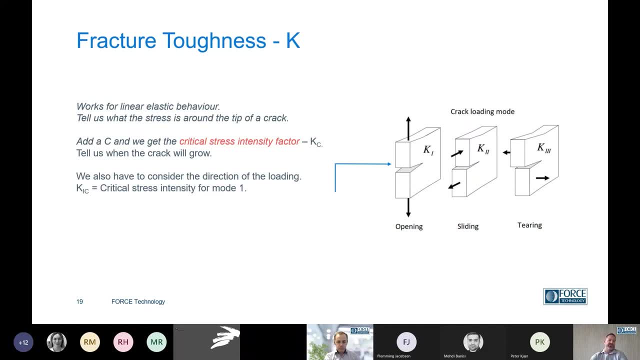 really you know, once it snaps, it snaps. you don't go into into a lot of ductility and a lot of uh toughness. so material with high toughness will not necessarily we won't use this type of testing, even though k can be part, as we'll see later, it can be part of it. 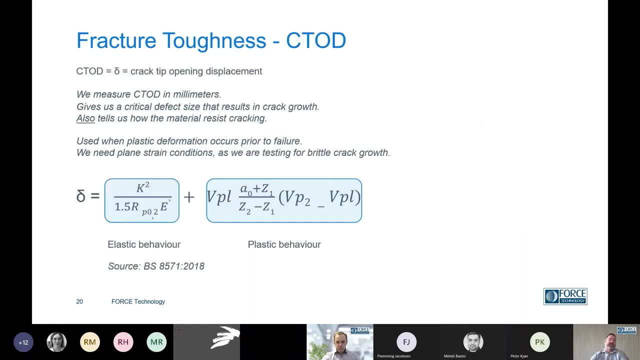 it's just the start. we then need to look at other things, and here we've got ctod, or fracture toughness, uh, the corrective opening displacement, and um, it includes plastic deformation. that happens before failure, so we have elastic plastic conditions. so the mathematics then has to include both the linear and the non-linear part, as we can. 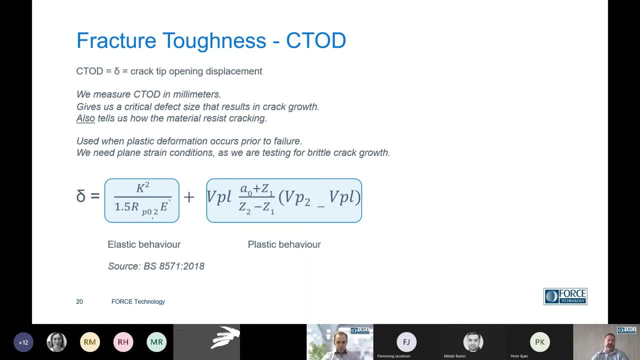 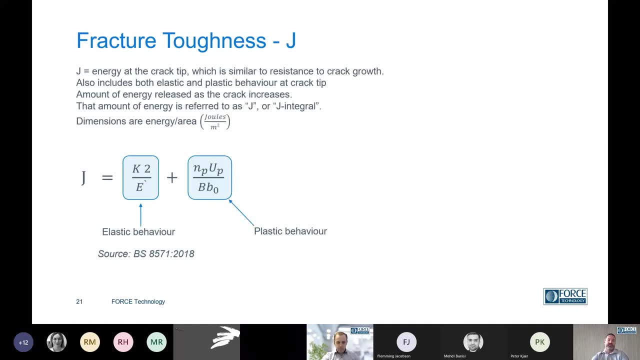 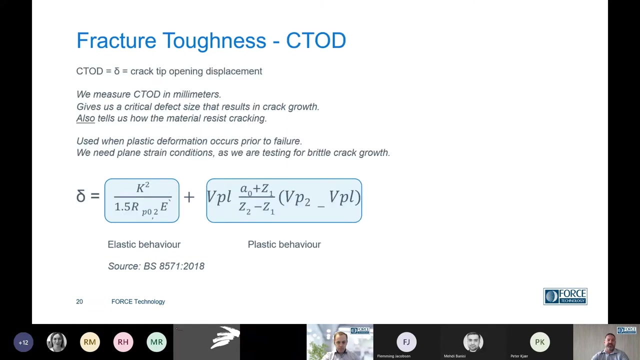 see there by those, those blue boxes. it gives us both, both behavior. now another one similar to ctod is the j or the j integral. this is not an objective one. it uses the force factor and peta, so j or the挺 will not twist as much as the protein does. so even though i said with 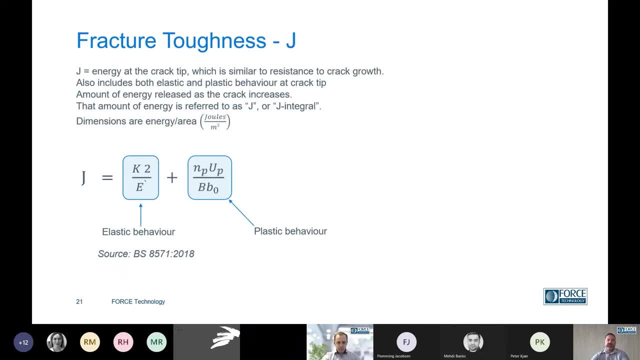 That's the way that the fracture toughness is derived- is different for this one. it looks at the energy at the crack tip, uh, whereas crack tip opening, displacement, crack tip opening, that more as looks at the mouth, how the mouth of the the crack behaves, where this one, um, even though it could use some of the, the similar equipment, its 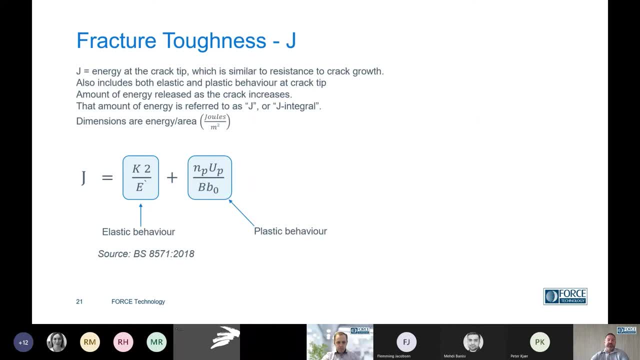 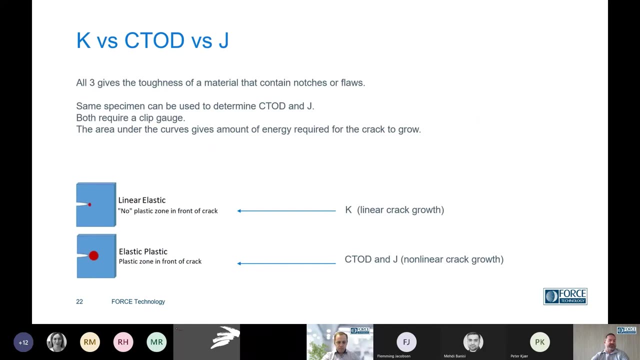 it uses the energy under the, under a curve, um, and the mathematics is different. so just a quick comparison of everything, um k and c to d and j or j integral, all three give the fracture toughness. now, uh, the same specimen can be used, um. we can add instrumentation to all of them to to understand what is happening at a very 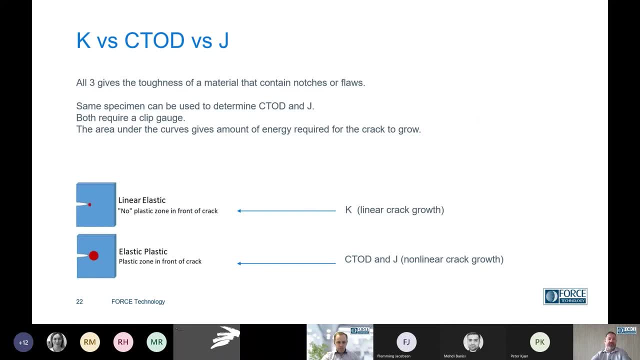 fine detail as as the crack propagates. but the key difference is that we've got linear elastic conditions and elastic plastic conditions. in other words, we've got uh, no to very little plastic zone in front of the crack, then we'll use k and if, if there is a a good plastic zone in front of the the crack, then we'll use ctod and j. 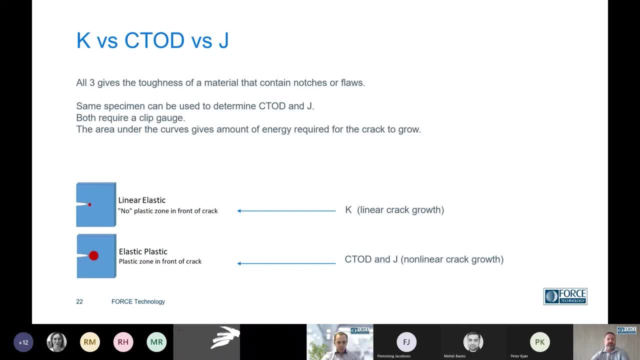 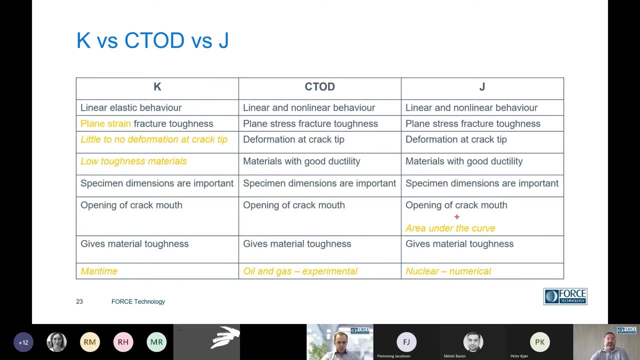 of course that's for the elastic plastic crack behavior. another way to look at this is a table. there are some- well, there are many- similarities, but there are some key differences. as an example, you know, look at the plane strain versus plane stress, or how the toughness is calculated and also where it comes from. 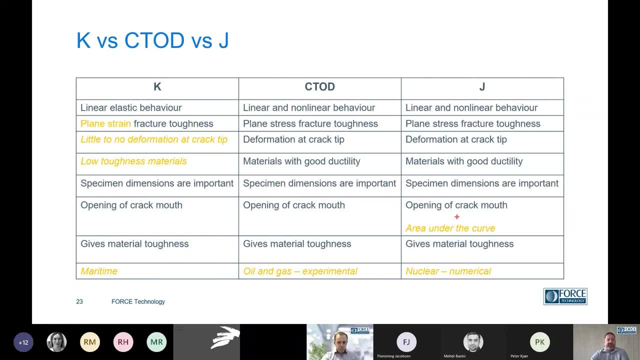 interestingly well, if you look at it at j on the right hand side, it includes the area under the curve. then for me, which is quite interesting is we can see that it's a little bit more Sexier, so the quality of the time trial is a little bit better. 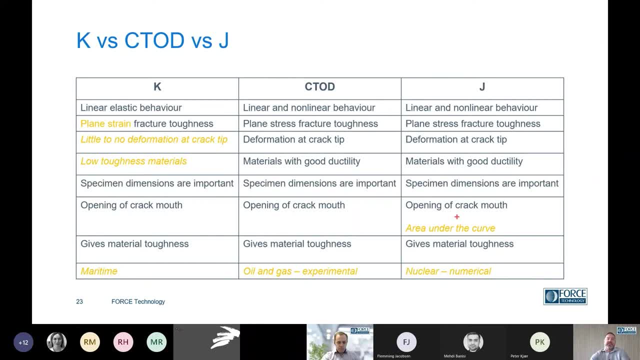 when you do that. so we have a. here's a little bit of a. you can see the fault in this slide, but the fault is a little bit more. it's not very much of a difference between the one that that we had in the world and the one that we have in j. 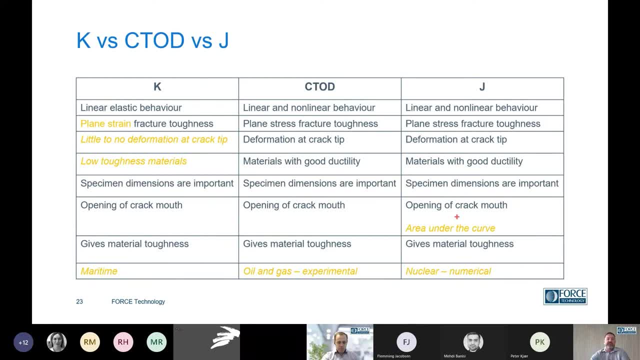 but the one that we have is called the shock stress factor, and what I get from this is the effect of the fraction of the force that I just showed you, that the weight of the fracture is much more thought out, and that is about the rate in which the to the area is applied. the 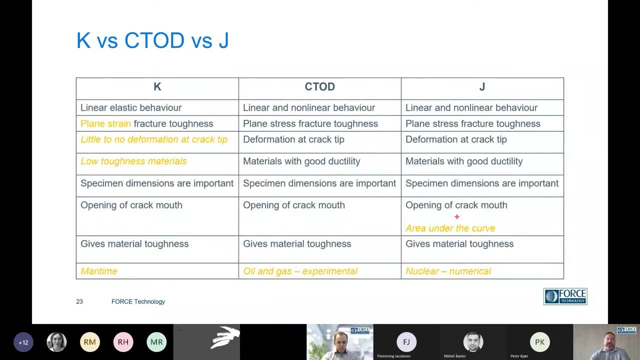 you can spot it here. it's a little bit of a burr: experimental ways to do that, while as the nuclear industry they relied on numerical methods. but of course it also relied. it also used the testing part, but their methods were more numerical than it was for the nuclear industry. 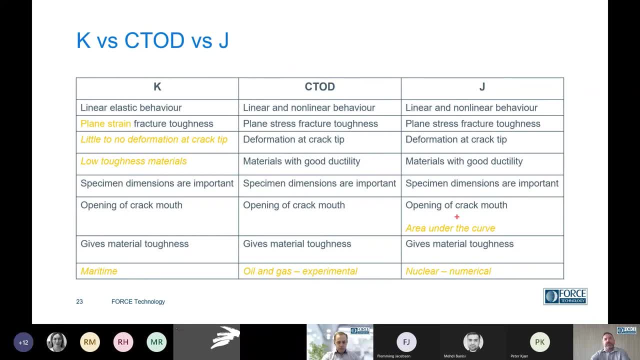 So what am I trying to say here, Apart from it being interesting? there isn't one test that fits everything. We have to assess the situation, we have to assess what it is we're trying to do and then from there we can look at the test specimen, the geometry and also the type of test, the type of loading and the type of testing. 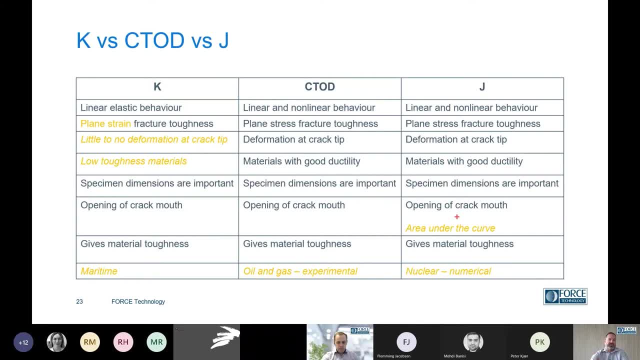 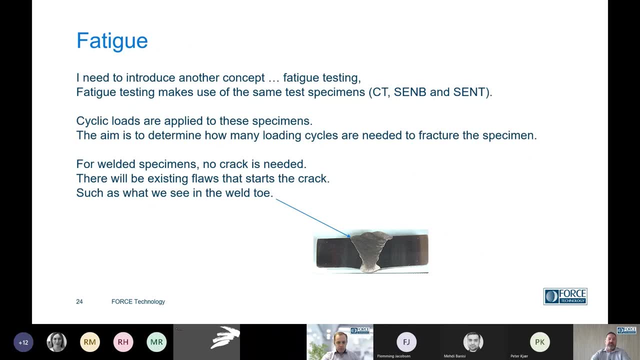 So there's a lot of equipment that we need to attach to do it and, of course, the geometry is important in all of that. Now I'm getting close to the end of the presentation and I want to introduce you to fatigue. 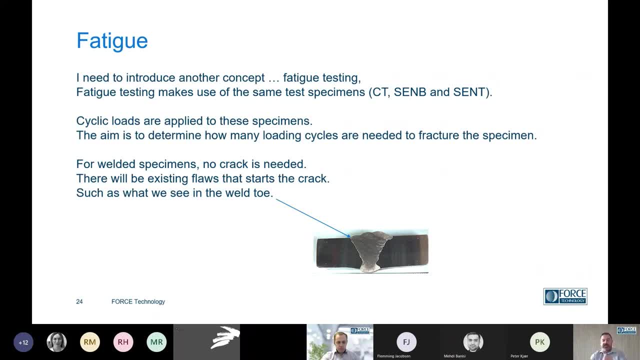 Now fatigue tells us how many times a load can be applied to a test specimen before it fractures, and luckily we can use the same specimens as before. But for welding we really have something similar to a crack if we just where the arrow is pointing the weld toe. 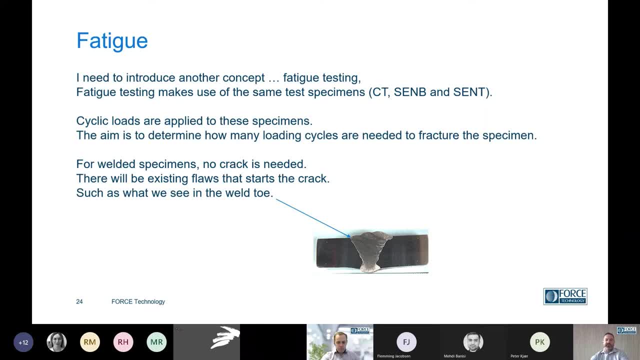 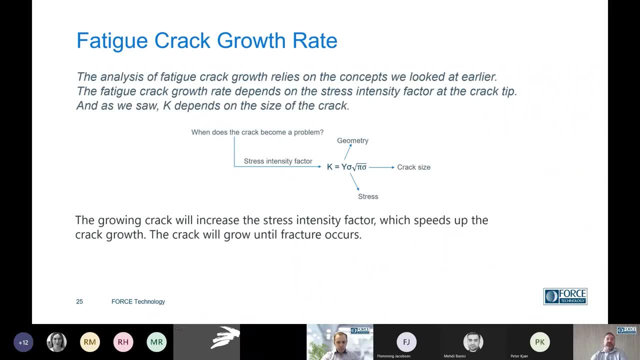 So these specimens may look a bit different, But the concepts that we looked at earlier- 4K and CTOD and J- those same concepts apply for fatigue, crack growth, The geometry, the crack size, the plastic zone and stress. all of this still applies and we can just copy and paste that over. 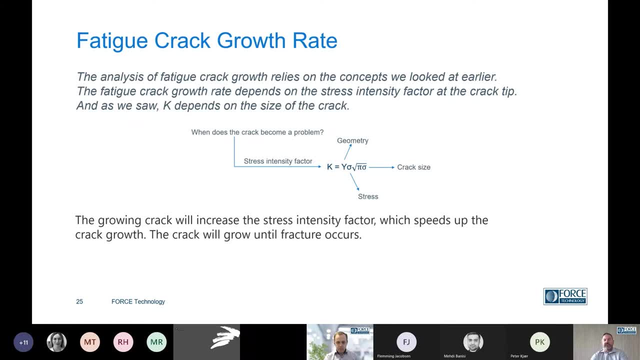 But something new to consider with fatigue is that the crack is going to speed up. You'll either have a phase where there's no crack and then it will start, and then it will be very fast and then you'll have your fracture. 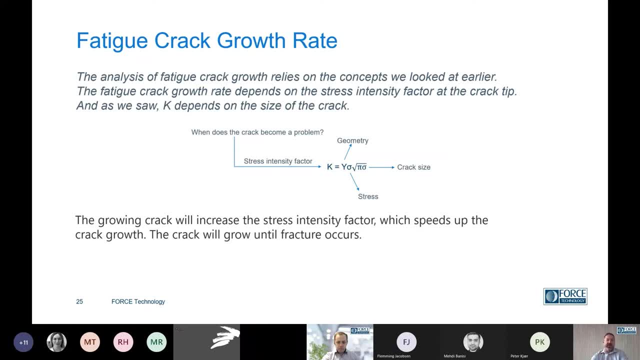 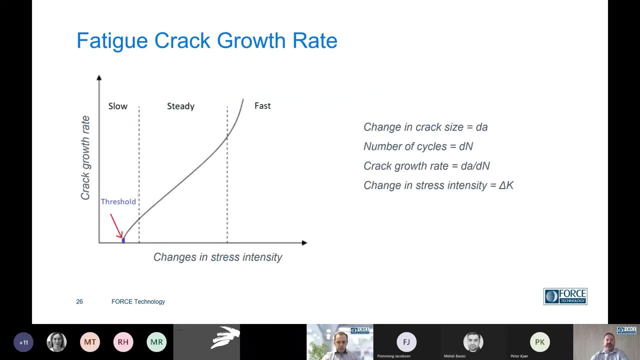 Okay, And it looks at what happens around the crack tip In that we've got. if we look at this graph, this- yeah, let's call it a graph- this curve here we see there's slow, steady and fast. 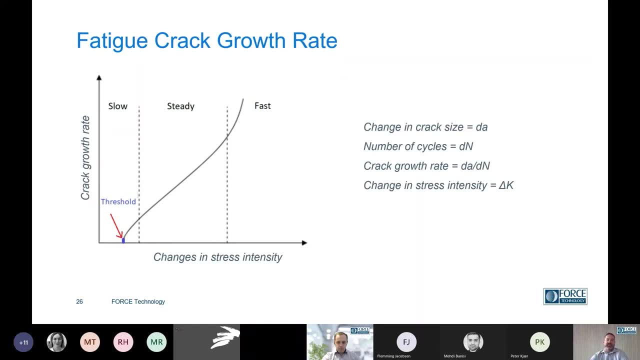 And what that tells us is that in the beginning there's going to be crack growth will be slow, Then the crack growth will be steady and then, towards the end, the last phase, it's going to be very fast. And another thing that we've got to look at is the speed. 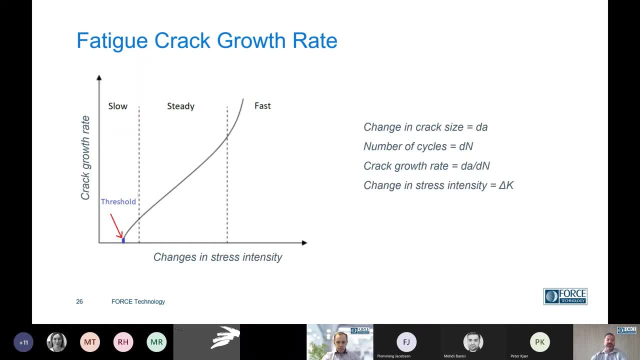 Another important thing: there is this red arrow which points at a threshold. Now, what this threshold means is that before this, the crack will not grow, regardless of how many cycles they are. It's just because the stress intensity is not big enough. 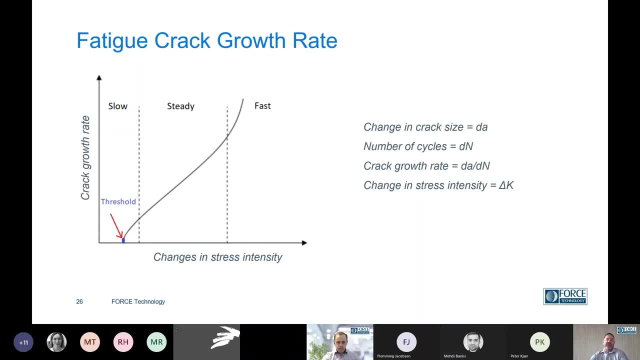 So this is one of the key things, important things from fatigue testing for fatigue. Okay, So fatigue crack testing is that to get an understanding of how it behaves? how does it go through these three phases- slow, steady and fast? 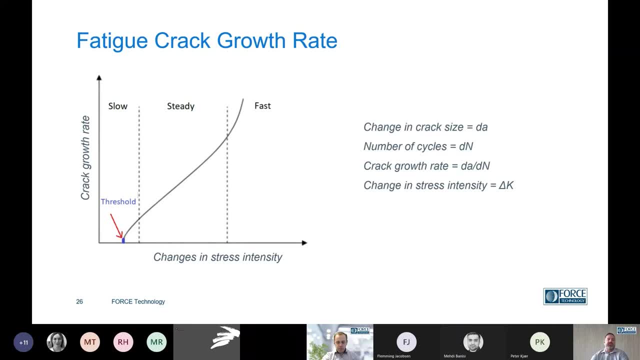 And what is the threshold value, What is the limit that we can set And say okay for this stress, and let's call it stress. for this stress and for these number of cycles, the crack is not going to grow. That's something that we can derive from testing. 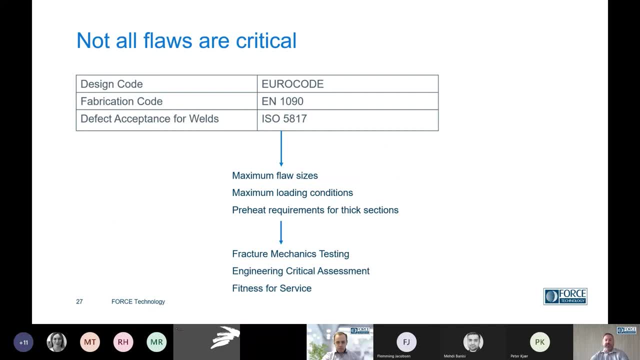 Okay, So I think I've come to the end of my slides. Hopefully it was very quick and it's a big topic and it's not possible in 25 minutes or so to put everything in there, But hopefully I showed something new. 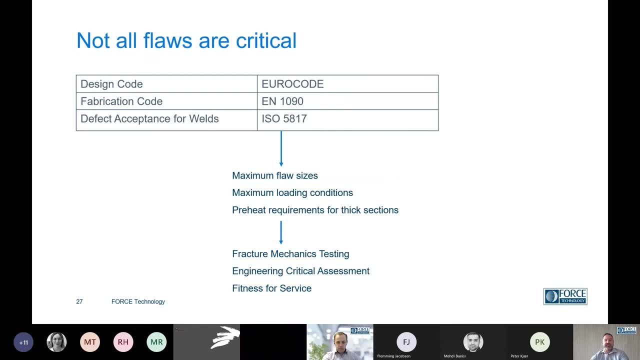 And hopefully I could introduce you to fracture testing, Fracture testing and fracture mechanics. If we have that information, then we can revisit the question that was asked in the beginning: Is there a safe way to deal with flaws? Do we just have to stick with the maximum floor size that is stated in the specs and in the codes? 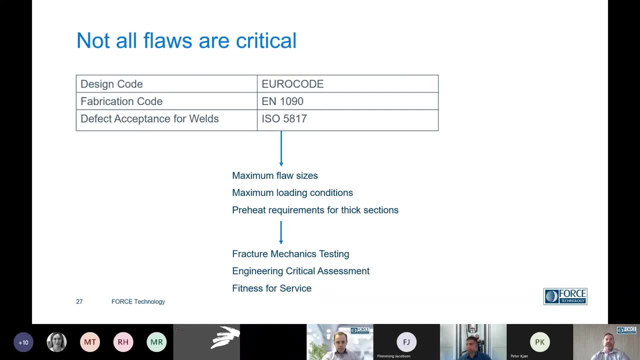 Or is there a way around it? What can we do? So what I introduced today is the fracture toughness and fracture mechanics approach, And luckily there is a safe alternative, And I will hand you over to Maas and he will then be able to tell you more on how we can do that. 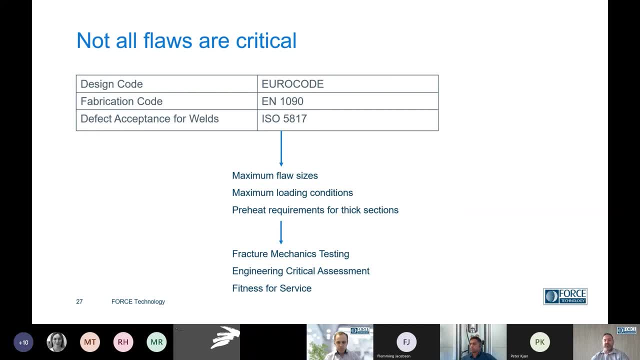 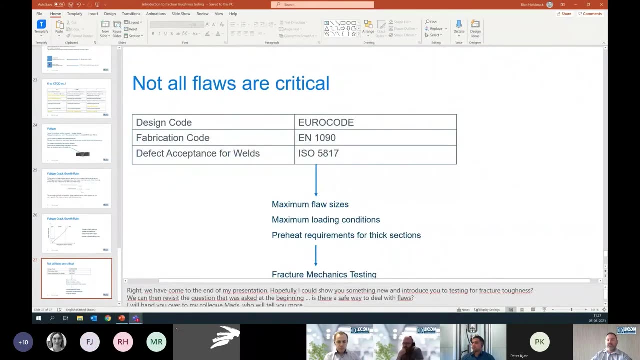 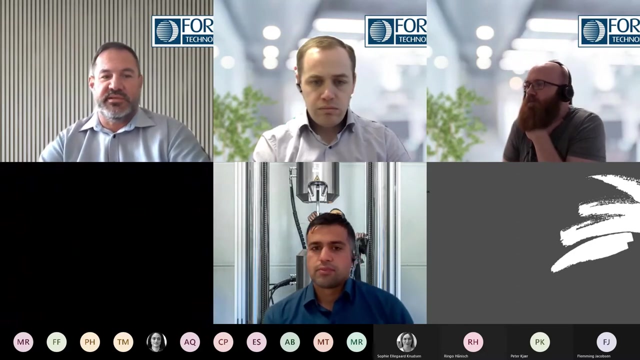 So, Maas, are you there? Yes, I am Okay. What I will then do is I will stop my presentation And all yours you can take over. Are we going to have some questions before I start? Oh yeah, of course. 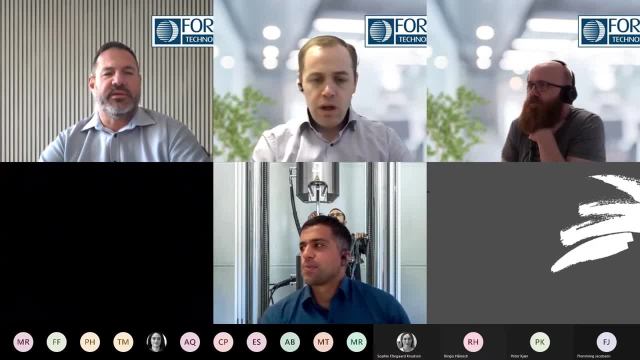 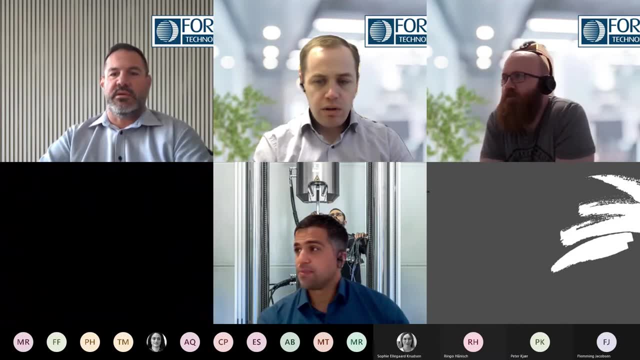 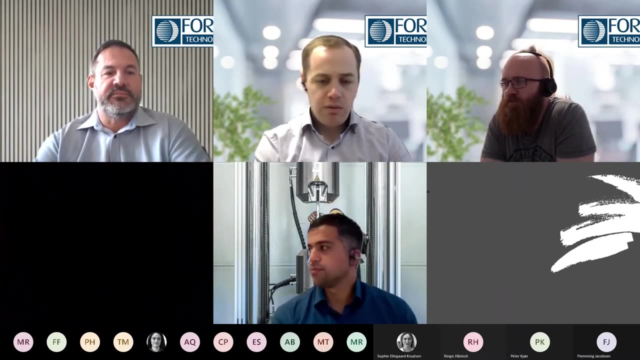 Eric wanted to have a break. Eric, Yeah, just because anyone. Rhian, I think you might need to mute me. Does anyone have any questions that came up from the first part of the session? I know Rhian and Maas might be able to pitch in here. 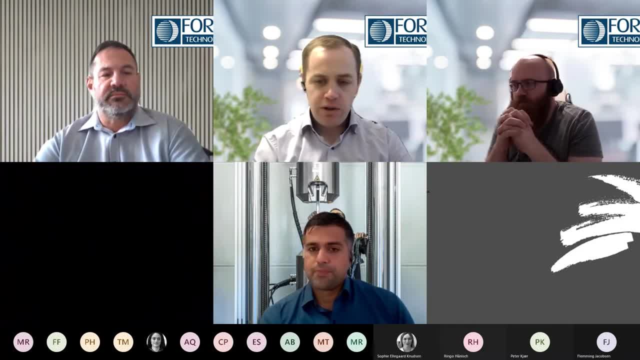 If we have anyone with questions, feel free also just to unmute and shout out. We're not that many people, So I think it's okay for us to start a little bit of a conversation as well. I would actually like to pitch in here. 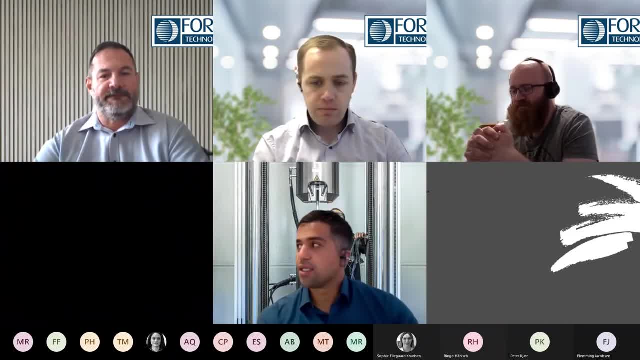 Rhian. thank you, Rhian. thank you for the presentation And I hope you can hear me. Yeah, I can hear you On the other side of Denmark. Well, actually, as you covered it quite well yourself, it's a very broad topic. 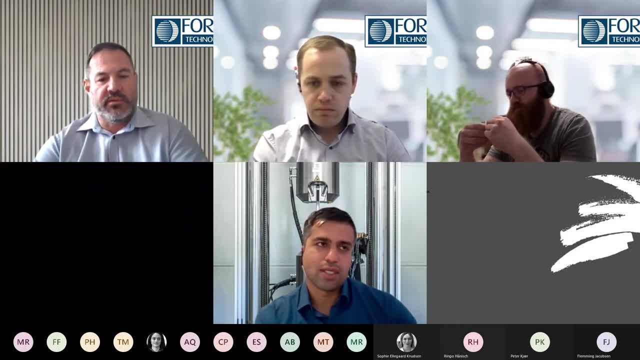 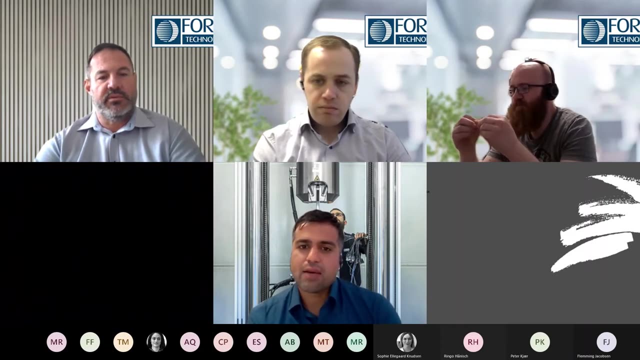 And you managed to give us a very broad look into it. And actually, before this webinar started, we actually got some questions, Some questions coming in And I was thinking if you could just take two of those before we move to Maas. 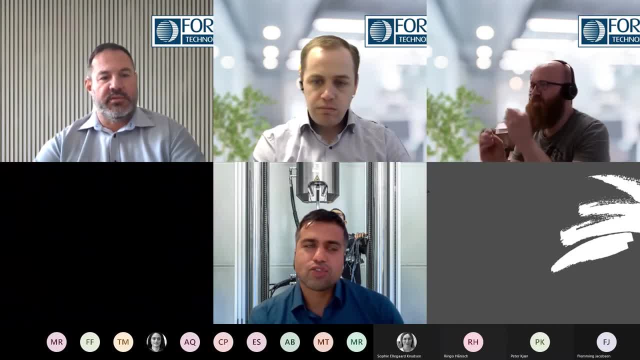 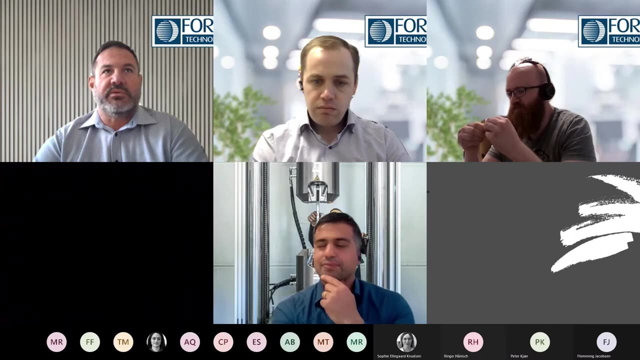 And there is one concerning the difference between stress and strain. Okay, A very- I would say a very- easy answer would be that Stress is what you do to the sample, So it involves the load and the geometry That's what you apply to it. 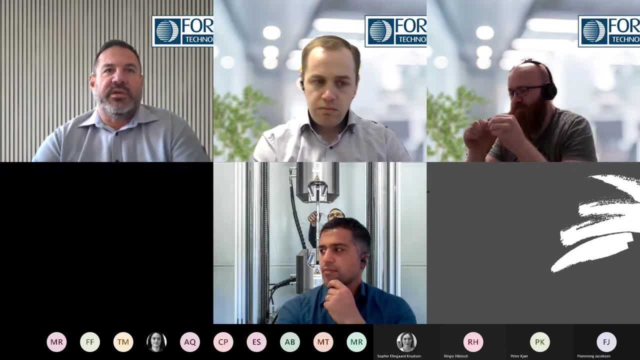 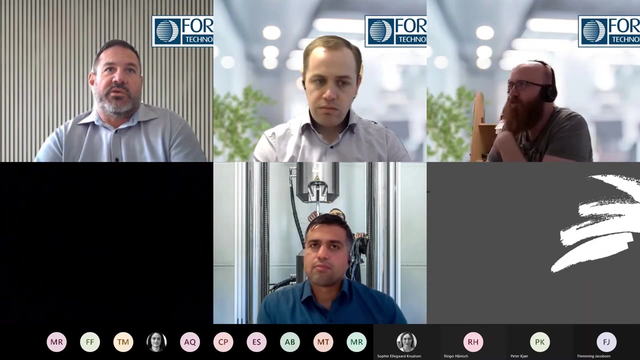 Where strain would then be how that material behaves once the stress is applied. And to make it even simpler, you know stress is what you do to the material, And then strain is how does that material behave once it feels the stress. So how does it deform? 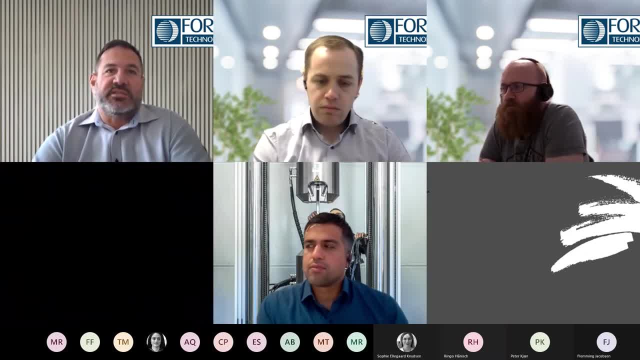 How does it change its structure? That is strain And stress is what it feels. So, in short, you would say that stress is the loading and the strain is the deformations of the material. Correct? We also may actually just have a. 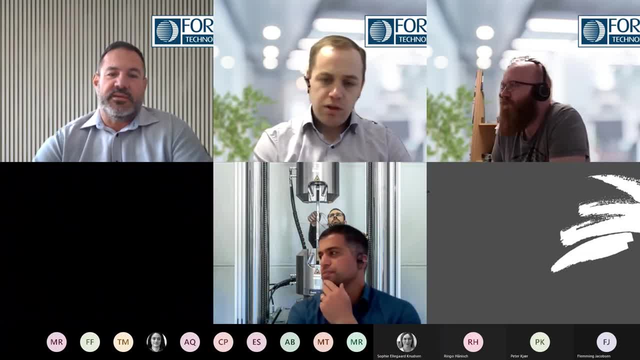 Question in the chat now, Yeah, Which is Rin. is it essential for the mounting points of the specimen on the upper and lower fixtures to have a 90 degree orientation against each other? Does this apply for all geometries? I guess it was something that was shown on one of your slides. 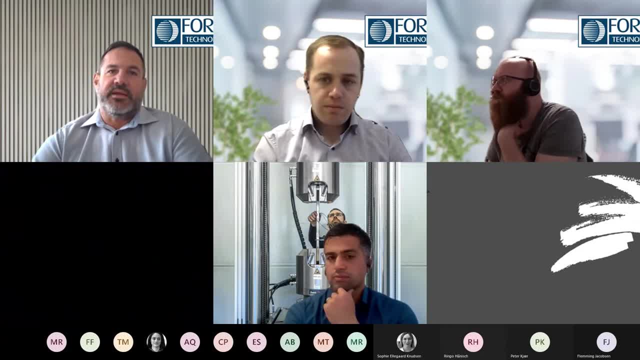 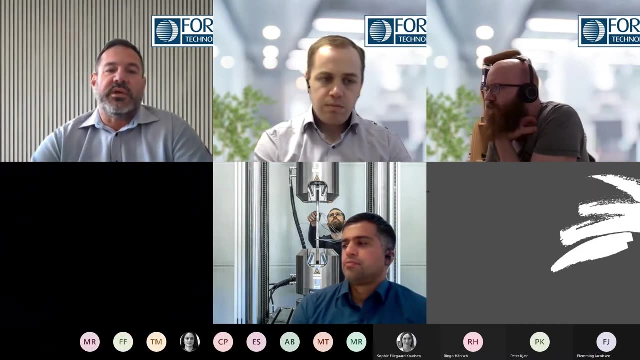 Yes, I would say it does, because it It depends on the test. Mads, help me if I say something wrong here. But what we, If we want to just simplify it, what we want to produce is: we don't want to introduce something at an angle, because then the application of the loads may not be symmetrical. 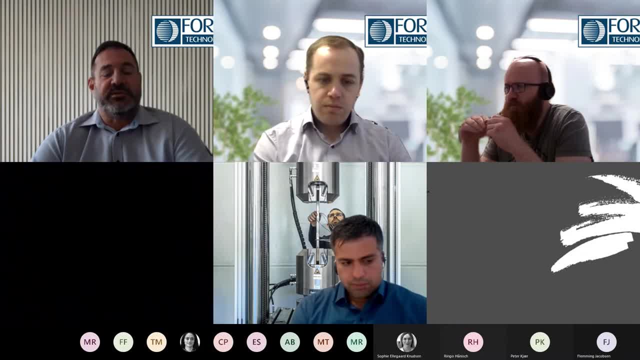 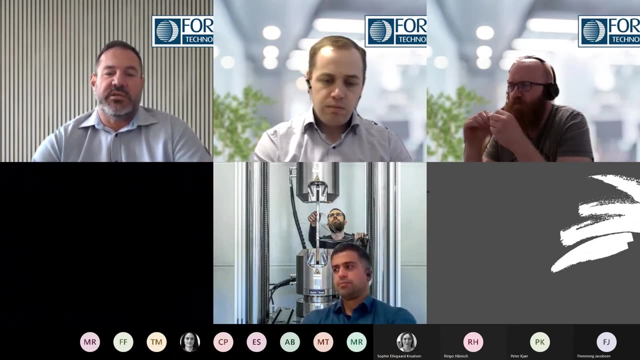 So from that perspective it's important that it is 90 degrees, But of course there will be exceptions, depending on the geometry of the specimen, Depending on what we will achieve, what we want to achieve. But I would say in principle, yes, first approach is make sure that everything is aligned. 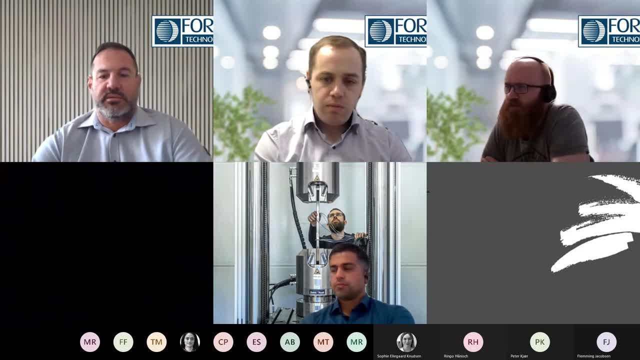 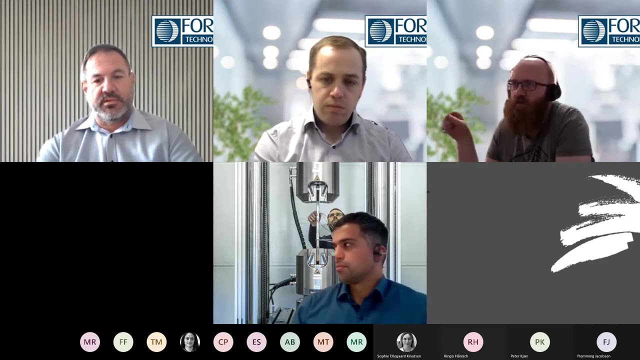 Yeah, There are different tests for fracture mechanics, So different setups, But most of them they introduce some kind of bending for the CT specimen or the SENB specimen And that requires the 90 degree angle in the way that the crack is oriented. 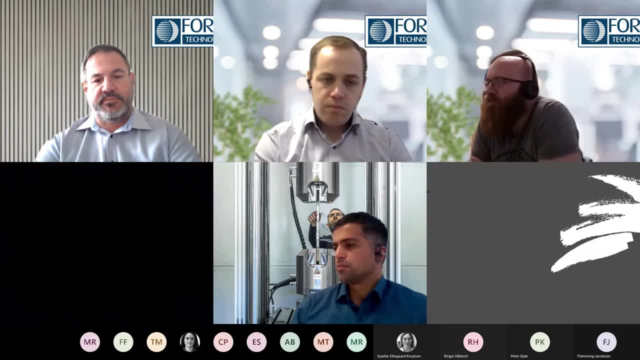 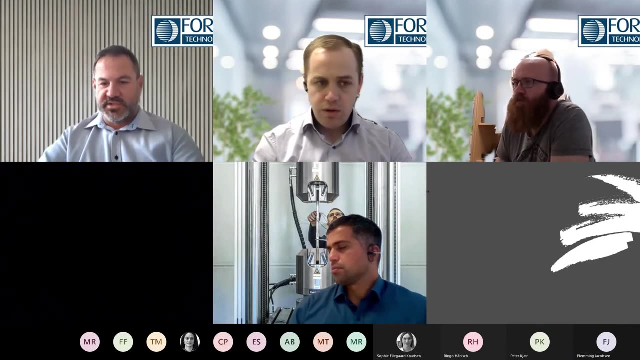 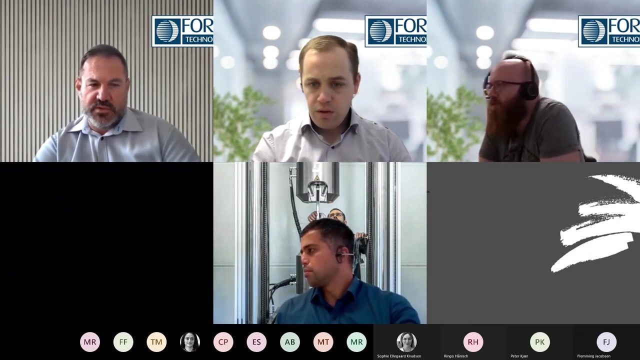 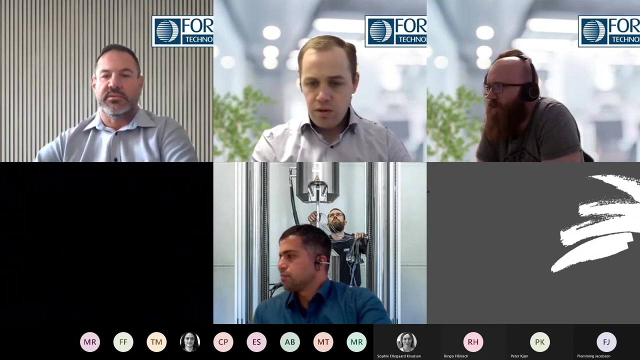 So yeah, So there's a question there from: Okay, We have a few more questions. Mekti, do you want to ask those questions? Can you see them? Or shall I do it So I can take the one for the fracture toughness, if it's better to increase the size of the specimen until getting it through the E399, not to switch to E1820.. 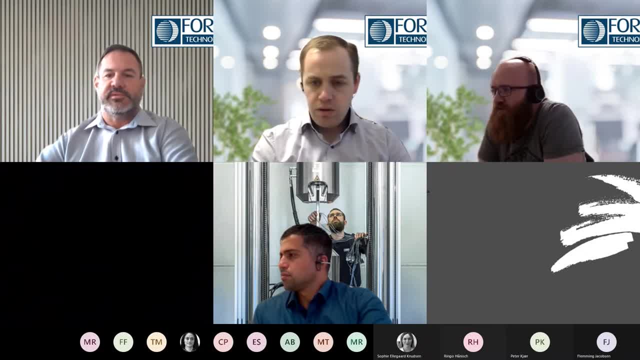 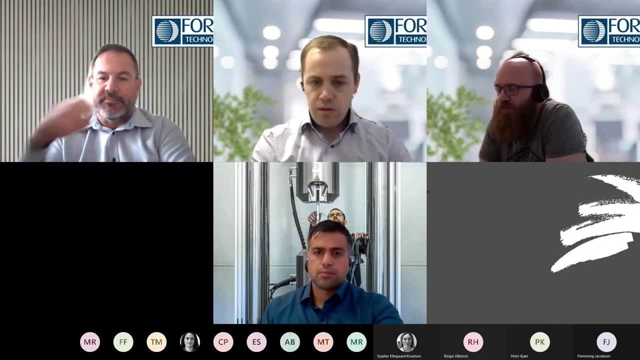 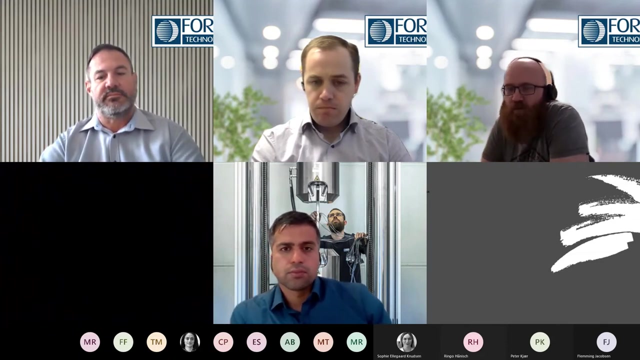 I would say that. I would say that sometimes, or very often, it becomes very difficult to get valid results in the K1C testing at room temperatures or zero degrees Celsius. When you're going to lower temperatures, then it is more, It becomes more probable that you will actually get a brittle fracture. 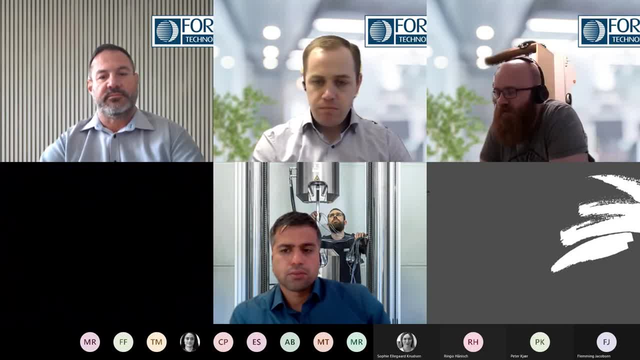 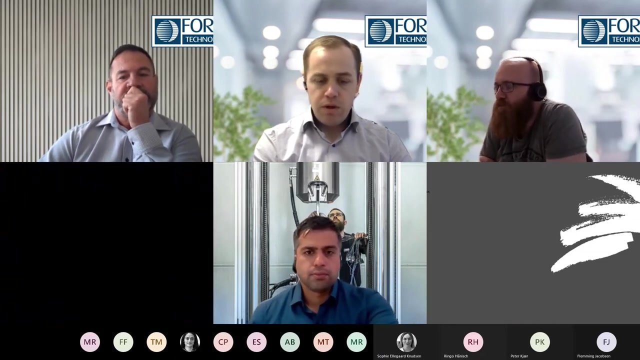 But In higher temperatures you will get unreasonable large test specimens that will not be able to fit in many test machines. So I would switch to the E1820 standard and do a CTOD or J-test material, Mekti. I think for the sake of time maybe we should move on. 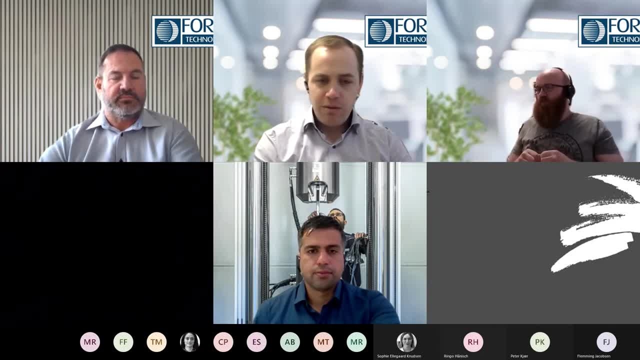 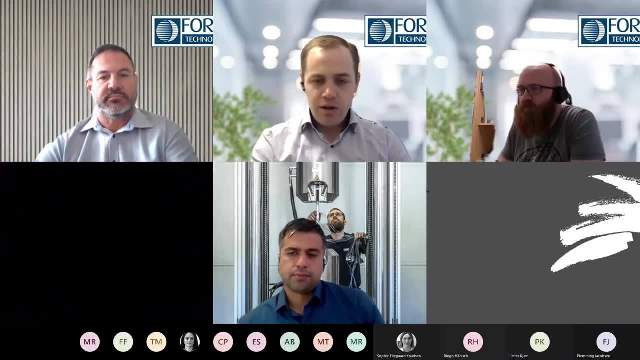 Since that question came, you know, via email. we can hold it to the end, probably, And for the sake of time, we should probably move on and let Mass run through his part. Yes, So, Mass, why don't you share, and we're looking forward to it. 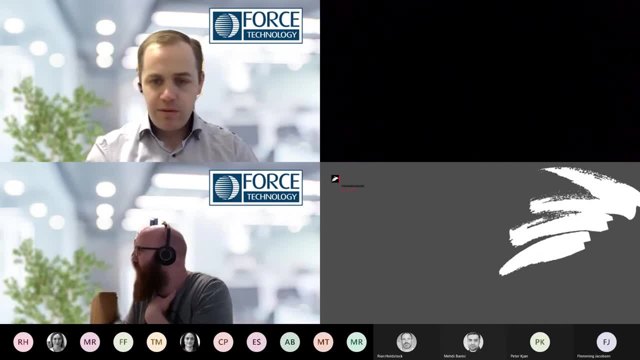 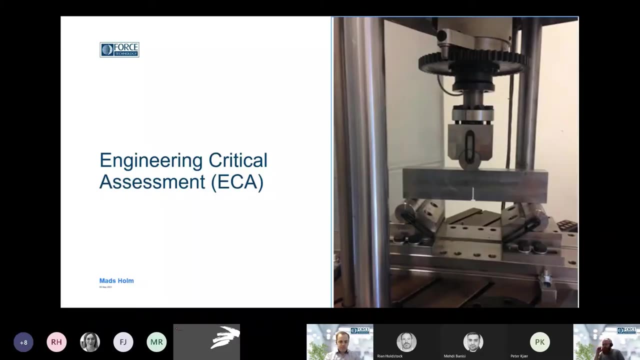 Will do. Just need to click the right buttons. Yes, I'm going to talk a little about engineering critical assessment. So that is, the assessment of floor sizes in structures And how we can estimate critical floor sizes based on the BS7910.. 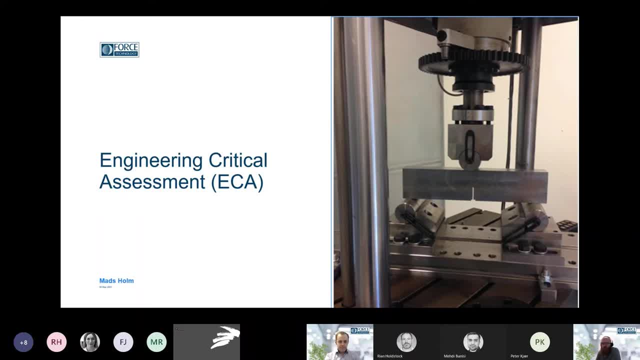 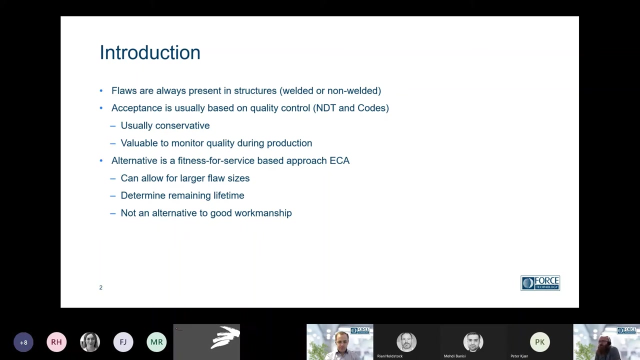 And also Actually using traction mechanics, testing to get some more, To increase the allowable floor size at least, And to estimate the lifetime of a structure with a floor. To begin with, just have a short instruction: Floors are always present in the structures. 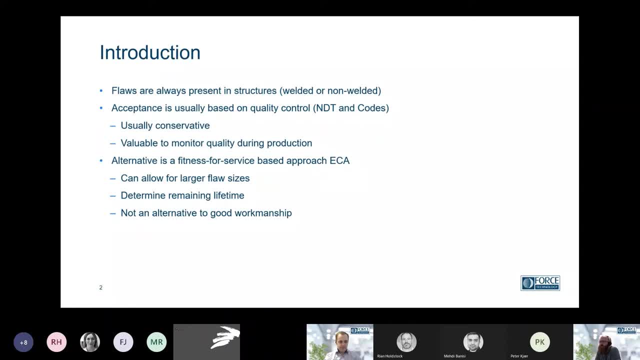 Yes, They are always present, Whether they are welded or non-welded. The acceptance is usually based on quality control. So that's using entity methods and using some codes that give some acceptance criteria for the For the floors that has been found. 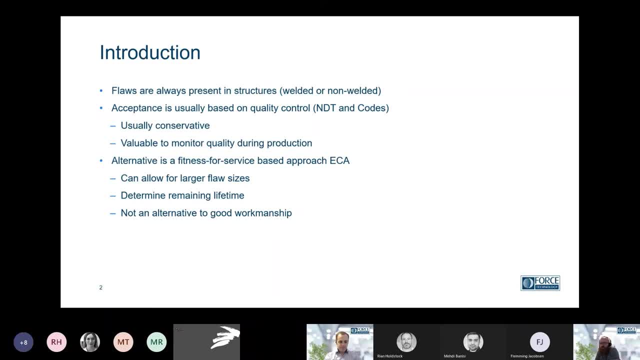 Usually these codes, they are conservative, So they are based on. Well, if the floors are Defects or indications are smaller than what we Say in the code, Then you should not have any problem with the The structure in its lifetime. 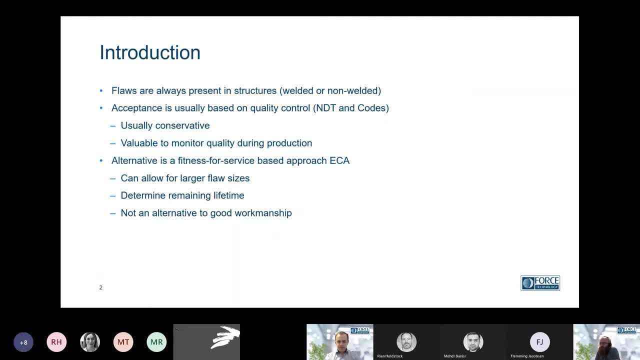 The entity and the codes. they are valuable to monitor quality during production. So that is just to make sure that the workmanship is actually pretty good for the things you are manufacturing. If you have defects or indications that are larger than what is allowed. 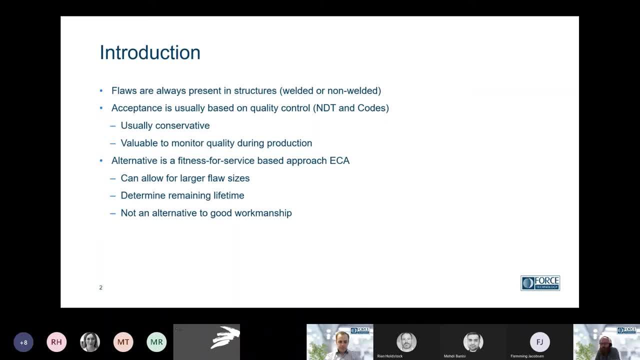 There is an alternative to Actually assess if this, If this indication is okay or not, And that is the engineering critical assessment, Which is a fitness or service based approach. This can allow for larger floor sizes. You may be able to determine the remaining lifetime if you have the 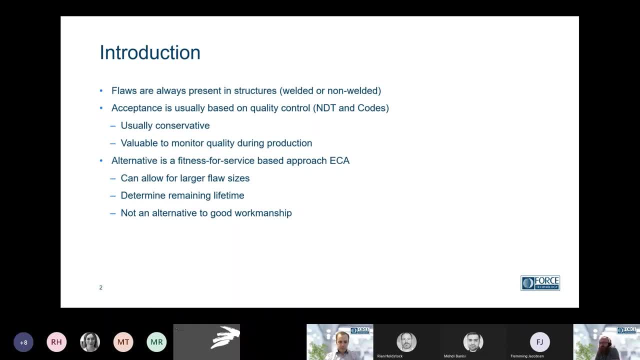 If you have fatigue loads, So you can estimate the crack growth during a lifetime. But Again, I would say that this is not an alternative To good workmanship. So if you are starting to have larger floors than are allowed for the codes, 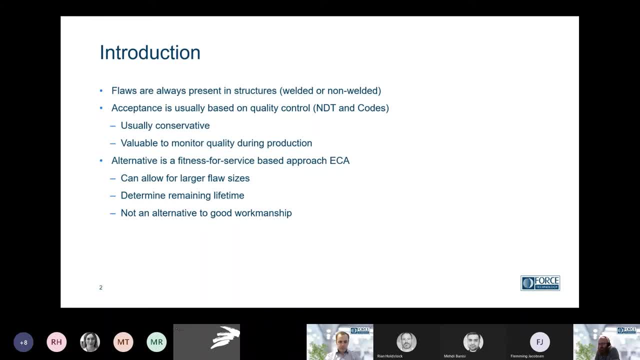 Then I would strongly recommend that you revise the production method And make sure that the quality increases, Because it is not just a way to say, Well, we can do the ECA and then we don't need to make good quality. So keep that in mind. 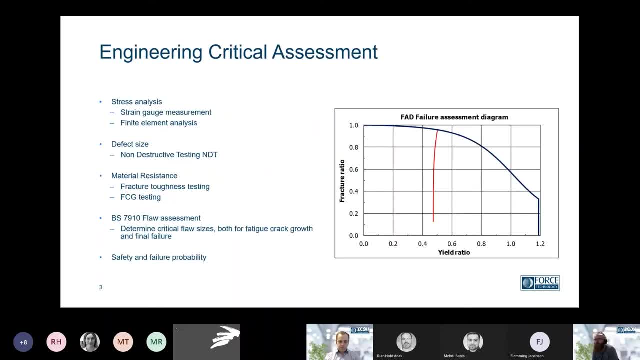 So engineering critical assessment. If we start to look at the fracture toughness Or critical floor sizes, On the right side of the screen you can see a failure assessment diagram And here we have the yield ratio on the x-axis And the fracture ratio on the y-axis. 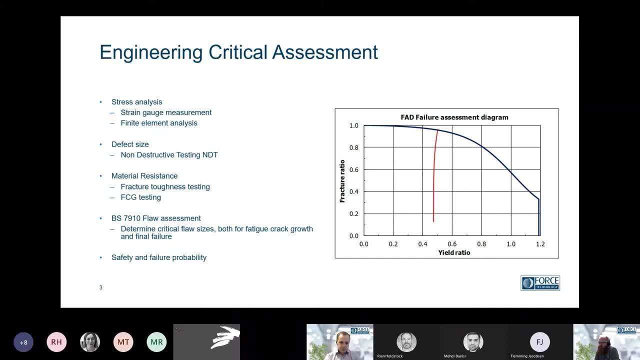 This means that we are assessing both for brittle fracture, That is, the On the y-axis, And then we have the yield ratio. How much of the yielding in the material have we? This is the y-axis And it's a combination of the two. 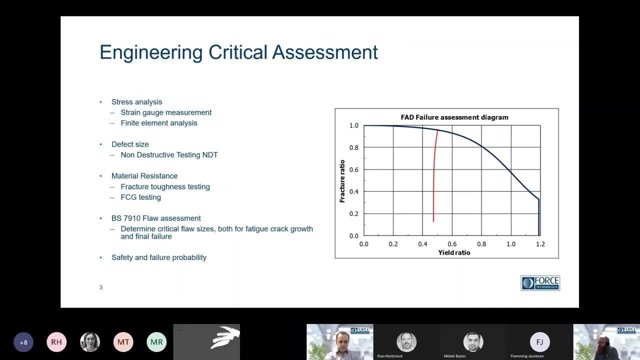 The area inside the curve- Blue curve- Is safe, And outside Then we have A risk of a fracture In the Floor size. The red line is actually an estimation of a beginning or a fatigue crack growth. So we start at the bottom. 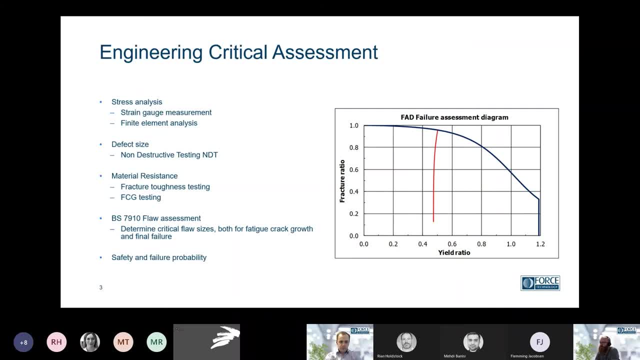 And then the crack growth Until it reaches the Failure assessment diagram. To do these Determination of the critical floor size, We need to do a stress analysis. It can be done by either string gauge measurements Or a final analysis. The defect size need to be estimated. 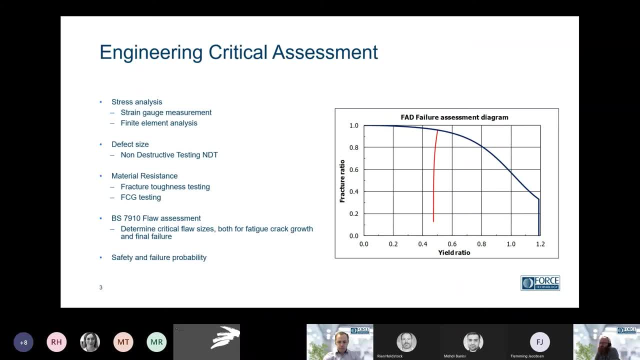 And that's usually done by non-destructive testing. We need to know the material Resistance, So again We can get that from fracture toughness testing And fatigue crack growth testing For fatigue crack growth curves And then we use the BS 79 standard. 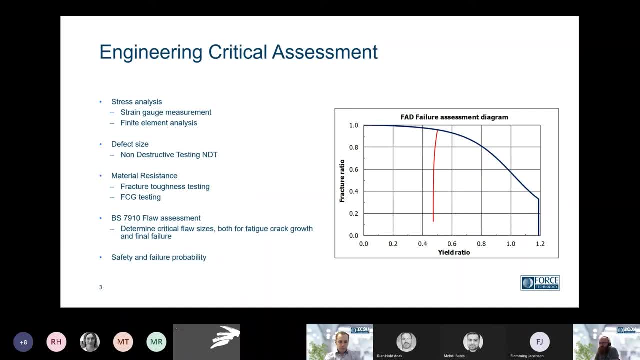 To do the floor assessment, And here we do determine the critical floor sizes, Both for fatigue, crack growth And for final failure. In addition, Safety and Failure probability May be necessary to To get The result that you can live with. 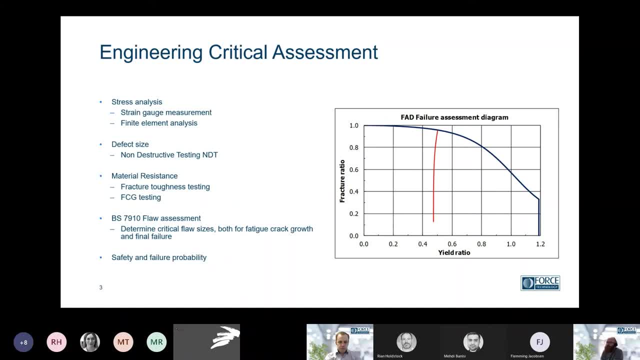 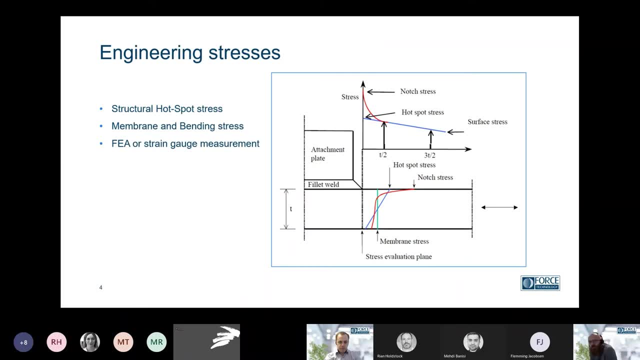 In the probability for a failure. So The engineering stresses we use in these Assessments It is usually the Structural hotspot stress. We use the membrane and the bending To measure stress Based on a linear stress Through the thickness. 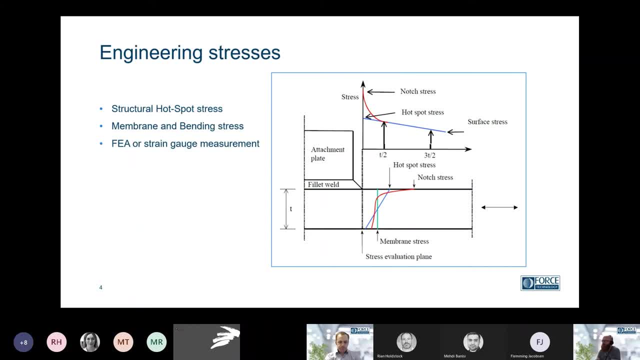 And again We can do this from finite element Or string gauge measurements And the On the Sketch here on the right, You can see, here we have Two points Where we have the measured stress And then we extrapolate into the. 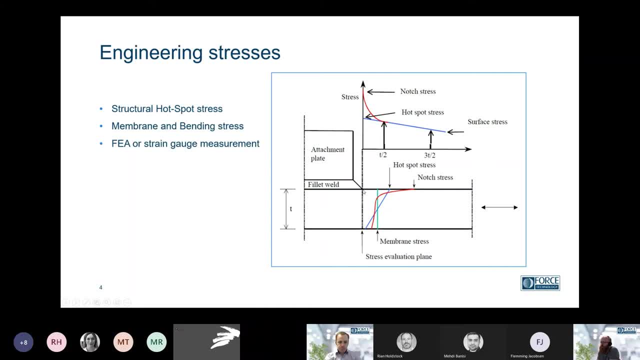 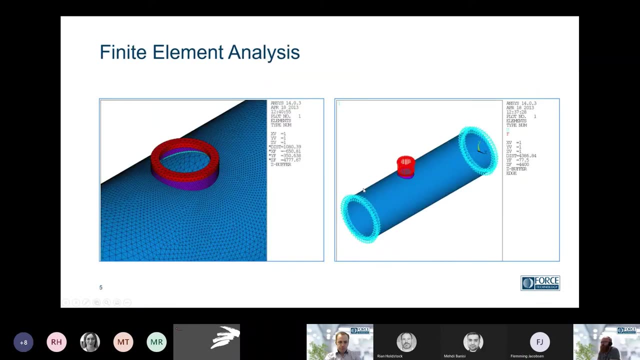 Point of this field world Where we want to find the hotspot stress, And here we have a Membrane Component And then we have the Bending component. The blue line, Green is membrane And the Blue is The hotspot bending. 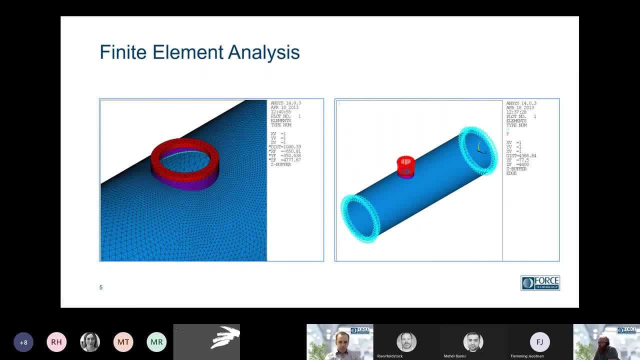 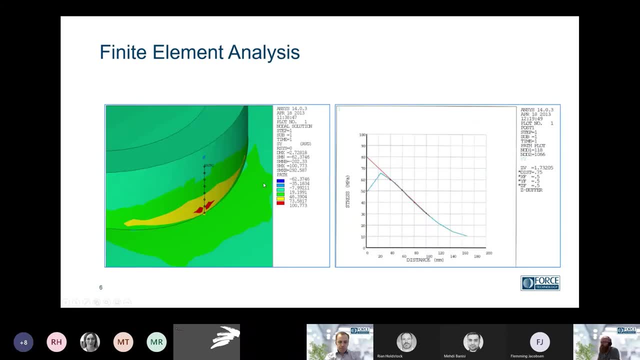 For a final analysis. It could be a Tube like this, Where we have Stresses applied And it's fixed in both ends And Here showing more, The way we estimate the stress Is again We. We try to get a path. 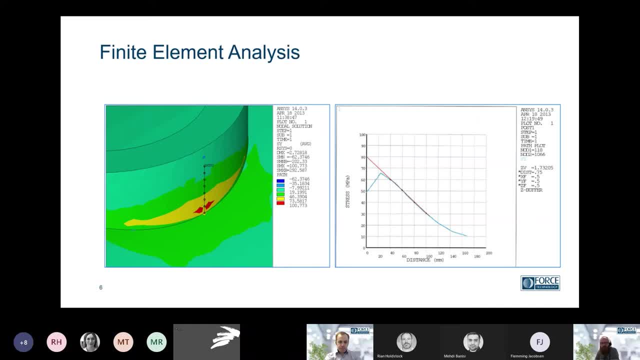 Up to the point where we have the Geometric Change And then we Estimate the hotspot stress In this way. So that's one approach With the finite element analysis. I'm not getting more into the string gauge As it is. 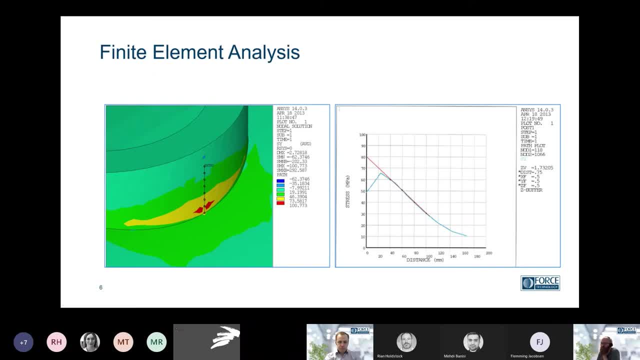 Quite similar, As you place the string gauges in certain Distances from the, For example the willow tail, And then you Extrapolate again The Two stresses Into the point where you Want to Find the stress. 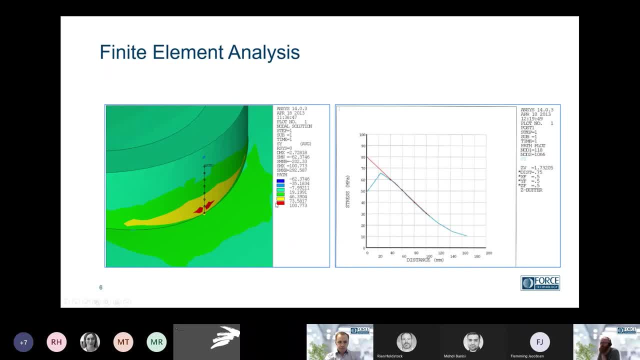 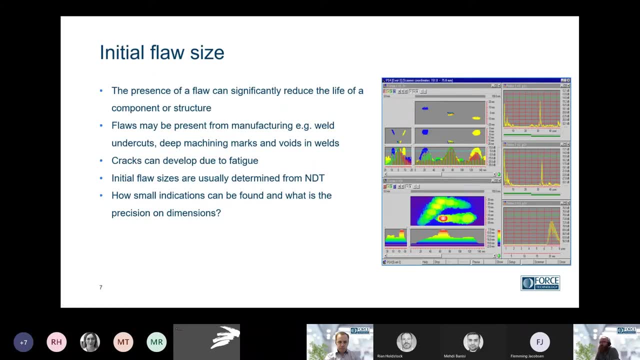 Next, We need to Know what the Initial floor size is. We know that the presence of a floor Can significantly reduce the life Of the common Component or structure. And The, The, The, The, The, The. 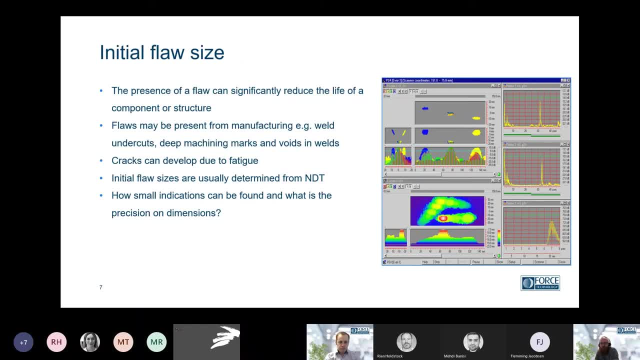 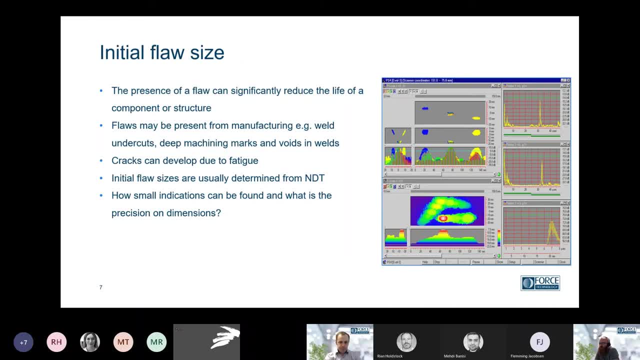 Foreign, The Jays, Previous, Yeah, The, The Have, Do, the, The, The, The, Their entity method. with a high enough probability that you will find them if that is 3 millimeters or 5 millimeters in length. 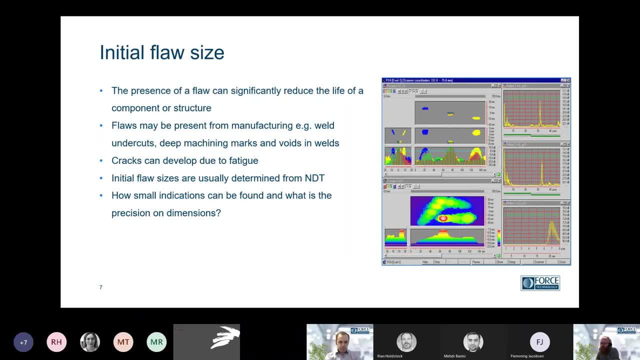 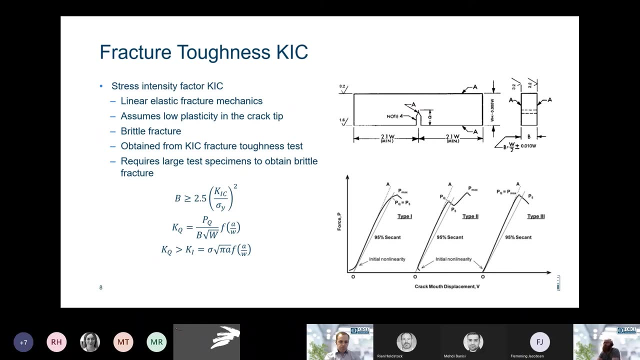 So there is again here with the initial flow size. there's some kind of uncertainty based on what entity method that is used and what is the probability of actually finding a specific flow size, Material resistance or the fracture toughness. I'm only going into the K1C due to time restraints. 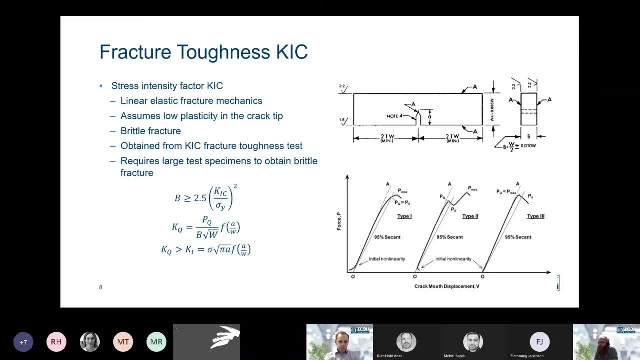 but K1C or K is the stress intensity factor And as we are also talking about, we are also talking about the stress intensity factor. What we're told is in the linear elastic fracture mechanics and we assume low plasticity in the crack tip and therefore we expect a brittle fracture from the testing. 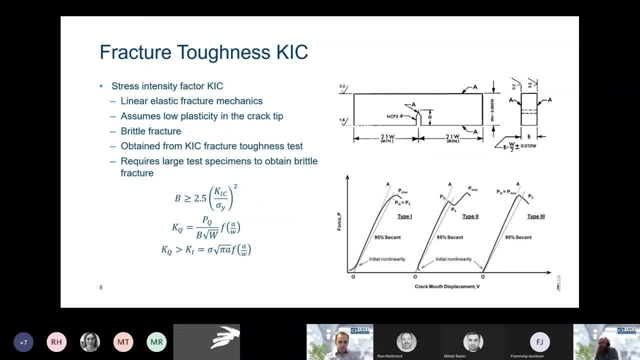 The K1C is obtained from fracture toughness tests and it has this downside that we also talked about here in the questions before, that it often requires quite large specimens to obtain brittle fracture And the ASTM E399.. E399 requires that the thickness B is larger than the two and a half times the K1C divided. 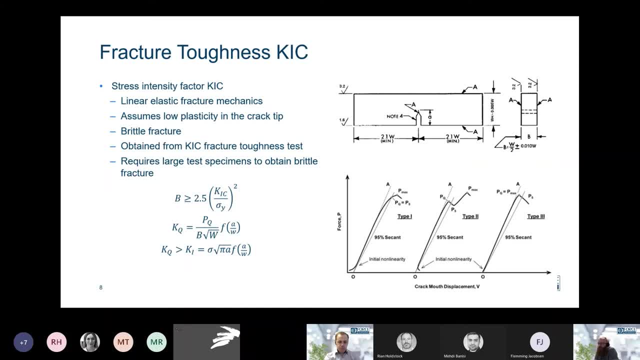 by yield strength in the power to two KQ or K1C, if it's a valid test- is then based on the load that you apply at the fracture And the, As you can say, PQ. if you look at the sketch over on the right, there are different ways. 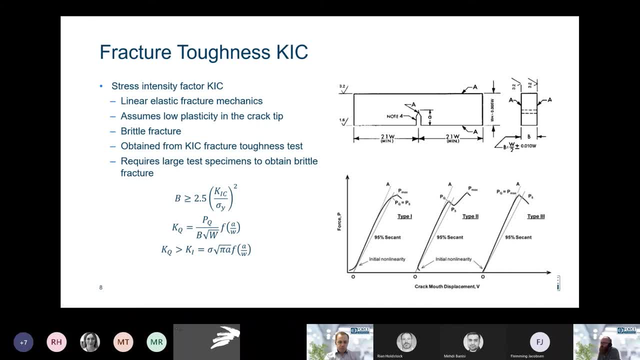 that the fracture toughness test can end. One is that we have a little bit of plasticity so we get some nonlinearity in the curve and then the PQ is based on the 95% secant line. here. If we have a pop in so there might be some porosity in the material, that actually makes 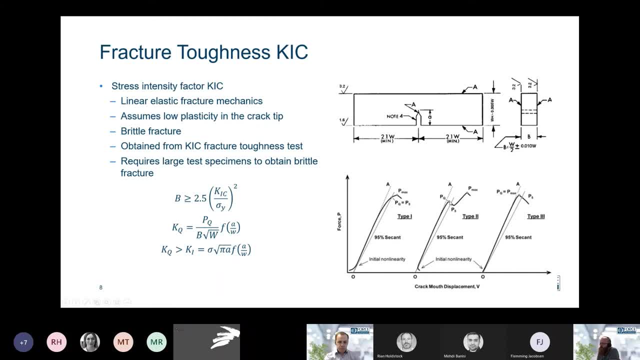 the, The, The. The problem is that The, The PQ, is based on the 95%, whereas the K1C is based on The, The, The equal to Pmax, where we don't have any pop-in and we have a very small plasticity in the material before fracture. 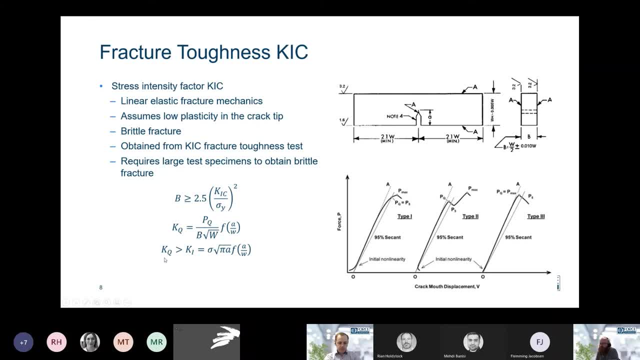 In essence, you can say that the tested Kq or K1c needs to be larger than the stress intensity factor K1, which is equal to the applied stress and the square root of pi and the frag height, a, and then a geometry factor F, which is a function of the floor size and the width of the plate, or geometry thickness of the plate you are looking at. 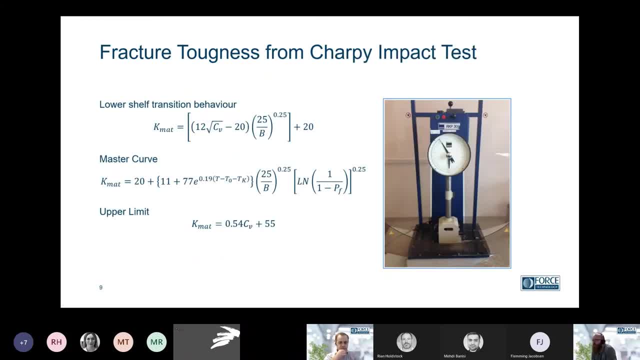 An alternative to fracture toughness test is that you can estimate the fracture toughness from a Sharpie impact test. This gives a conservative estimate of the fracture toughness. But if fracture toughness data is not available or it's not feasible to make fracture toughness tests, you can estimate fracture toughness from impact tests. 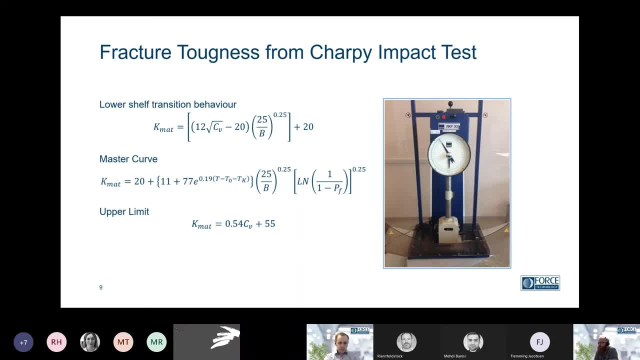 It is conservative, but it's better than nothing And it is used quite a lot, especially if it is structures that are already in operation and you can't get material to fracture. But you can get material from that to make fracture toughness tests And then you may have the impact tests from material certificates. 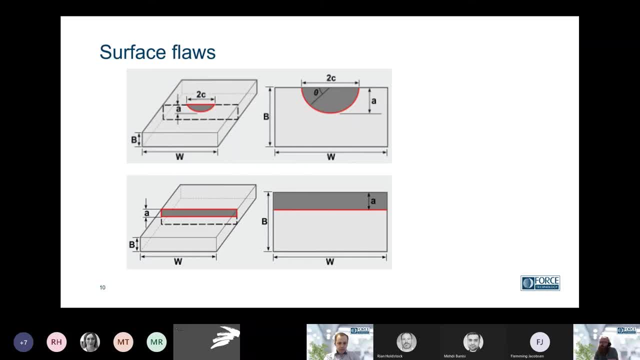 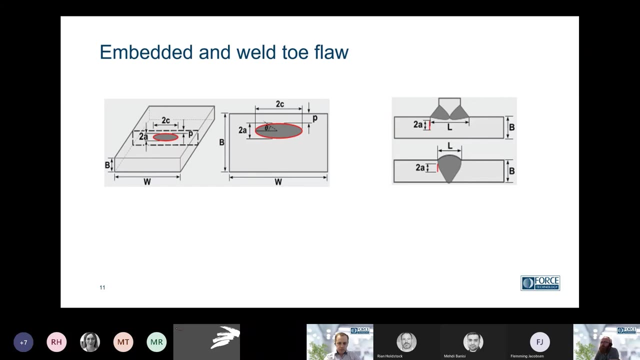 Then we need to know what kind of a floor we are looking at, And I will just show a few examples. We have the surface floors, A small surface floor on the top. We have a long surface floor here on the bottom. We have embedded floors which are inside the material. 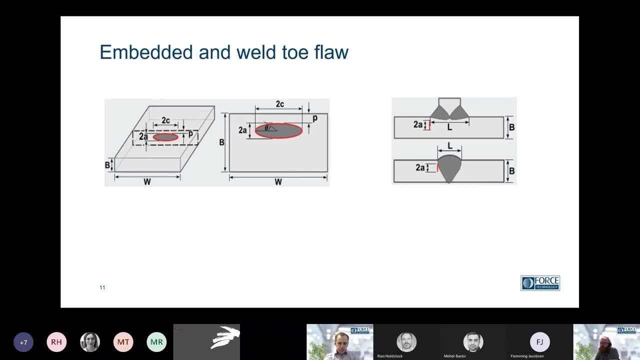 These are less critical than the surface floors and in my experience they allow for larger fatigue lives and you can have larger embedded floors than you can have surface floors. And then also if we have some floors near the weld toe, then we also need to account for that. 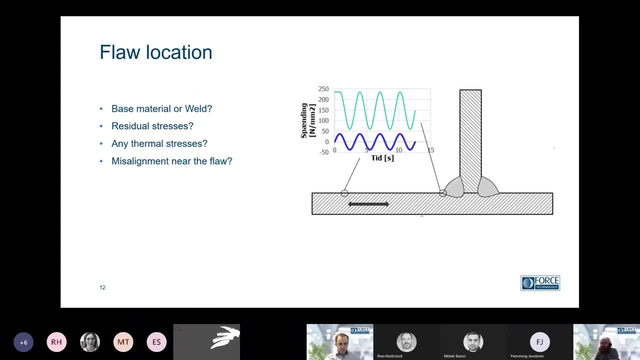 The floor location also has an effect on the size of the. We need to know if it's in the base material or near a weld, And that's one thing is due to that. if it's near a weld toe, as I said earlier, we need to estimate the hard spot stress. 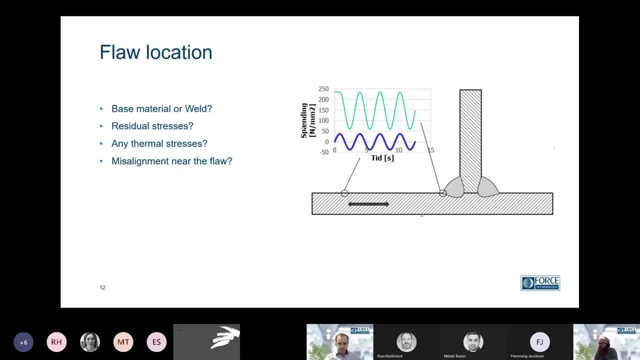 But also the residual stress is actually, Even though the material is Operating in a, For example, plus minus 50 MPa, then due to residual stresses, the Material near the weld will actually only have positive stresses. So you have a positive R-ratio. 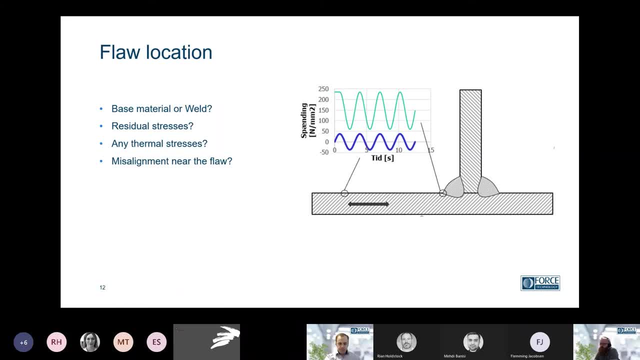 And that also affects both Your critical floor size, based on the fracture toughness, but also the fatigue crack load curve. if we are going to look into a fatigue crack growth, We need to consider thermal stresses and if there are any misalignment near the floor. 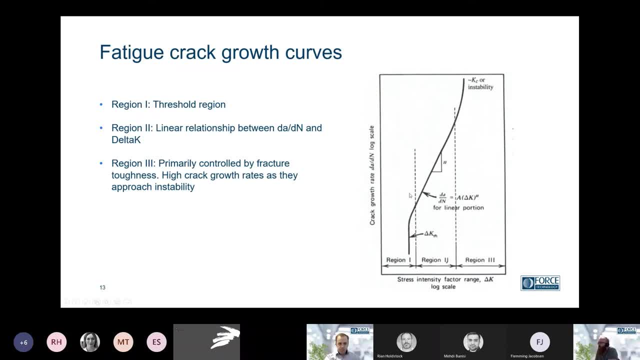 Rehan was also talking about this- The fatigue crack growth curves and the three regions. Or just say that the, The threshold value, is where we don't expect any Fatigue crack growth. Then we have a linear relationship between The crack growth and the delta K here in the region two. 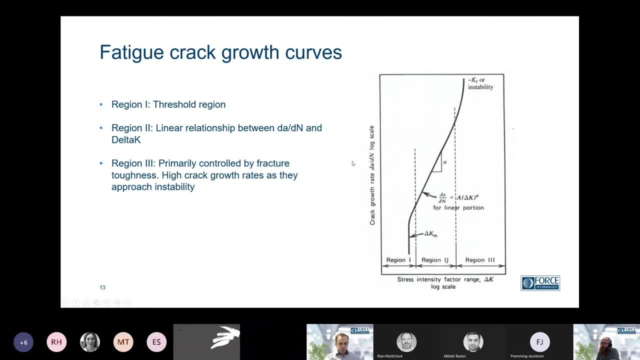 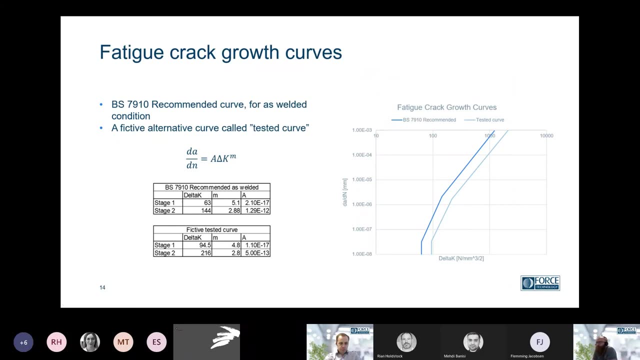 And region three. that's where we get instability and We are close to the fracture toughness in The delta K or the K value, maximum K. I'll go through a few examples, and For here I've used the PS 7910 recommended fatigue crack growth curve. 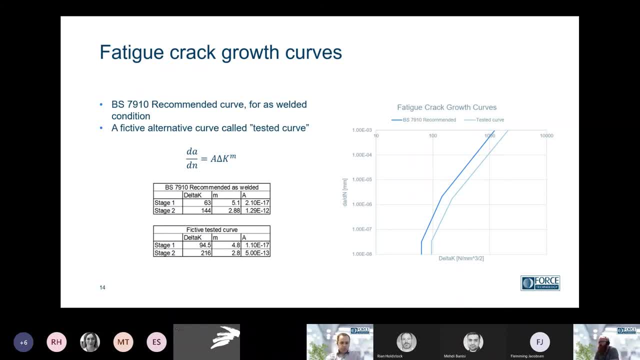 for, yes, welded condition, And I made a fixive alternative curve called the tested curve, where I've increased some of the values, both for the threshold value and the curve is a little to the right for the, Actually to the recommended curve. So it's just to show. 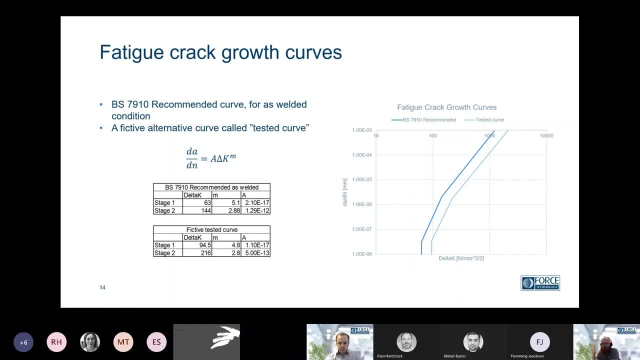 The difference And the possibility to actually use curves that we are Obtaining from testing. The relationship between the fatigue crack growth and The delta K is shown here With the GADN is equal to Constant A times the delta K to the power of M. 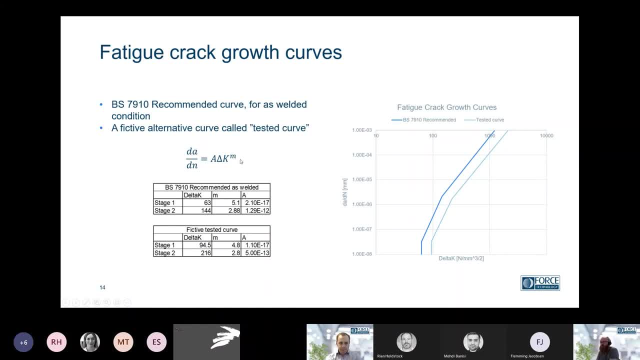 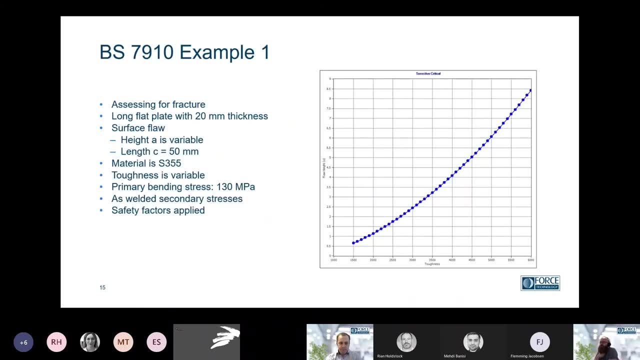 And the M is the Slope of the curve, you could say. The first example here is It's not on the fatigue crack growth, but more on the, The critical floor size. I've taken a long flat plate with a thickness of 20 millimeters. 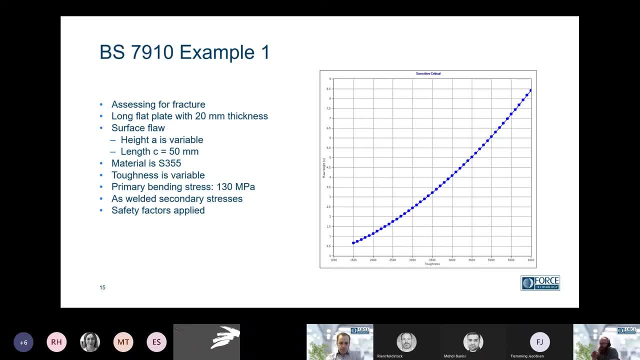 And the surface floor, With a height A which is variable, And the length C equal to 50 millimeters. The material is 355.. And The toughness is variable. So what you see here on the right is actually the Critical floor height. 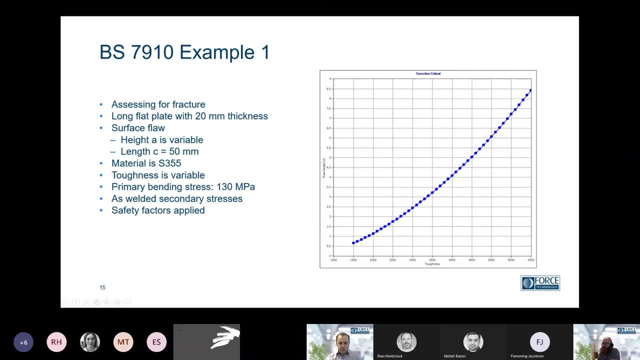 Based on the fracture toughness. The primary bending stress that I've applied to this Case is 130 megapascals. The condition is as welded In the secondary stresses And I've applied some safety factors on the fracture toughness and The size of the weld. 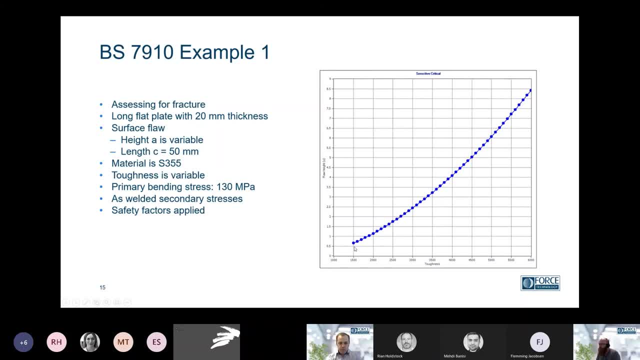 So, as you can see, When we, If the fracture toughness is around 1500 Newton per Millimeter, The power to three and a half, We get a critical floor height of 0.6 millimeters. If we increase to 3000 in fracture toughness, 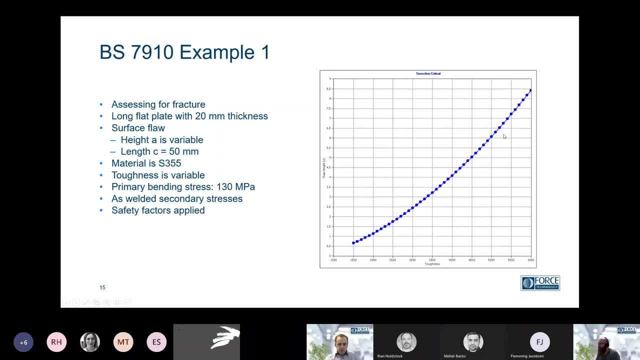 We have a two and a half millimeters, And If we go up to 5000, for example, then, As you can see, the Critical floor height actually increases quite a lot. The reason why I'm bringing this example is If we are using the 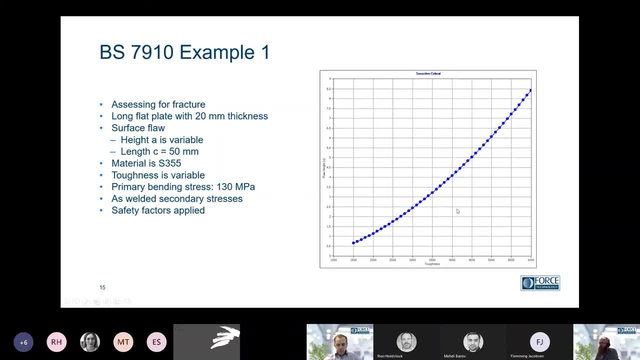 Estimation from Sharpie impact toughness. We usually will get some Values Between 2500. Maybe up to 2500.. But with fracture toughness test We might actually be able to get Higher values. So again, We can allow for. 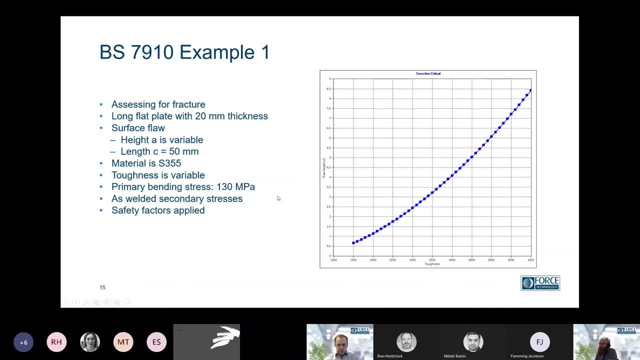 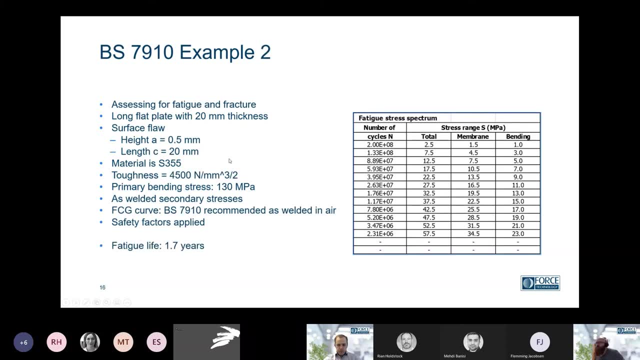 Larger defects which are not critical, or we can Increase the Lifetime of the structure, Which we will get onto here. in the example number two, Again, We have a long flat plate 20 millimeter thickness. I started with an initial 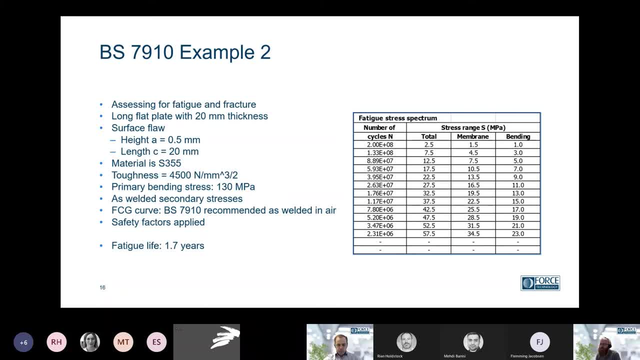 Surface floor with the height of 0.5 millimeters And the length of 20 millimeters. Material against 5 by 5. toughness, 4500.. Same primary bending stress And again We are in the As welded condition. 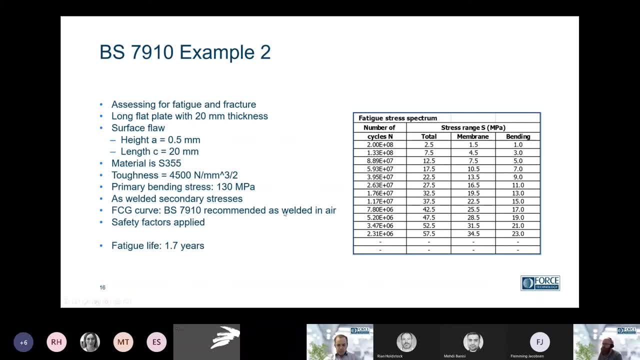 And for this Example I've used the BS 7910 recommended As welded in air curve. And again I've applied safety factors. The fatigue stress spectrum I've made up here. It's shown over here on the right Where we have. 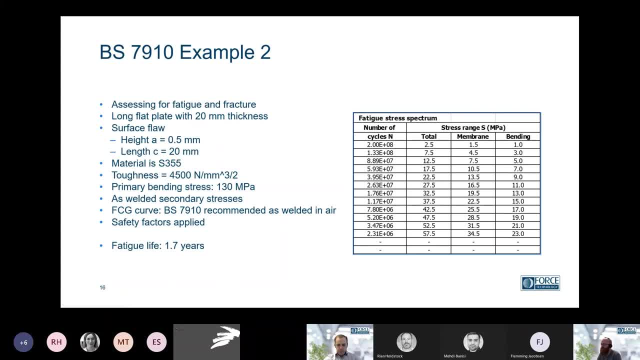 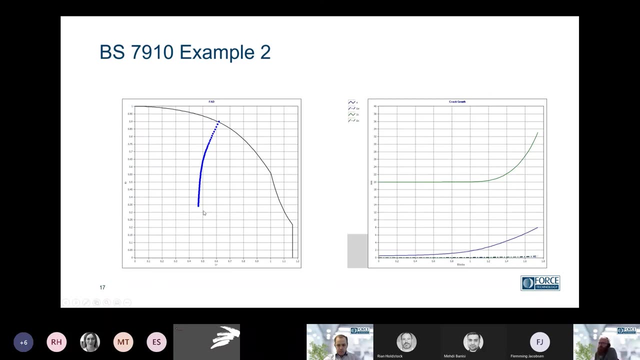 For This example is a 20. Estimated that this is a 20 year Expected Stress spectrum And the fatigue life here is 1.7 years, So shown here on the failure assessment diagram You can see The first iteration. 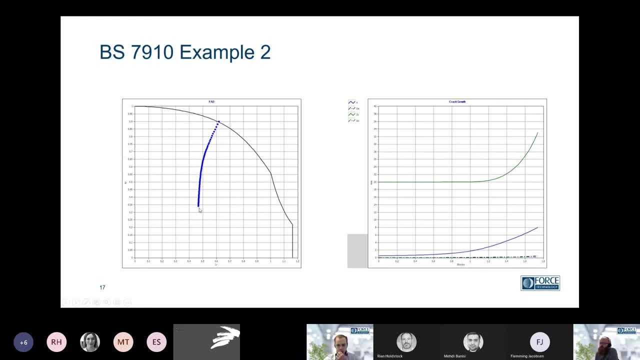 We are down here with the, The floor size And the floor increases in size, And then we reach the Figure assessment diagram curve And We have a Risk of a failure. Looking at the crack growth, We can see Both the 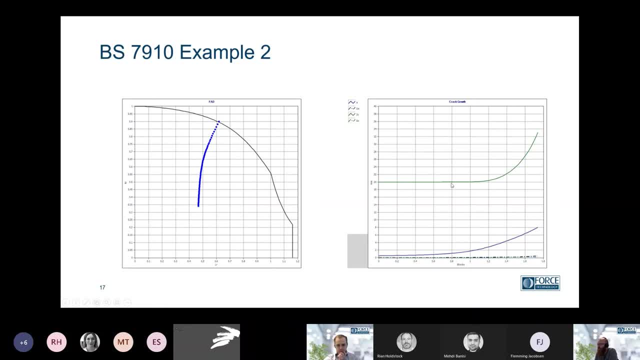 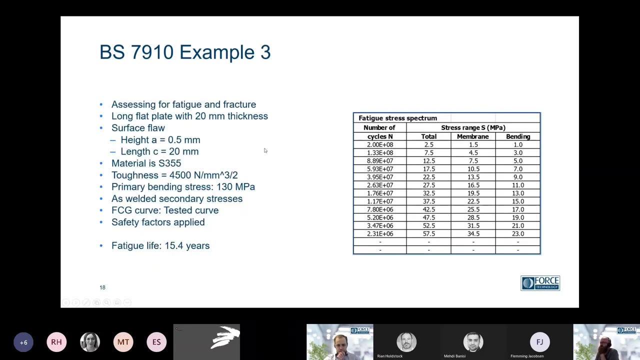 Floor height increases And the Floor length increases Until A height of 8 millimeters Increase from 0.5 millimeters After 1.7 years. The next example Is the same as the one before, But I've used the. 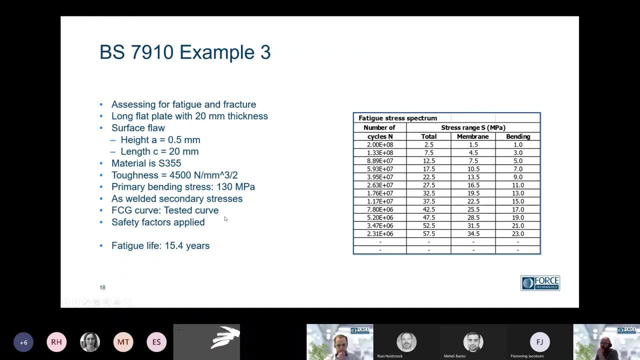 The as tested curve I showed earlier Where we had increased both the threshold And the fatigue curve was a little bit better. But the fatigue life here is increased to 15.4 years. And again You can see the same failure assessment diagram. 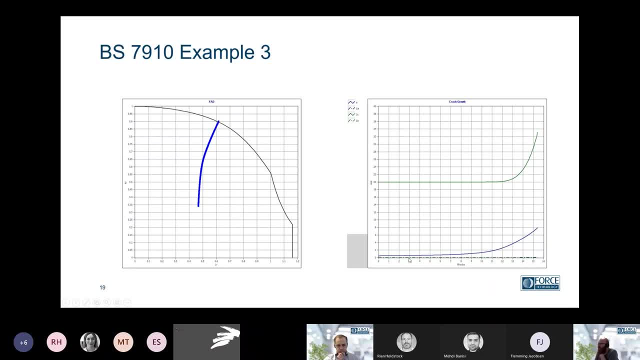 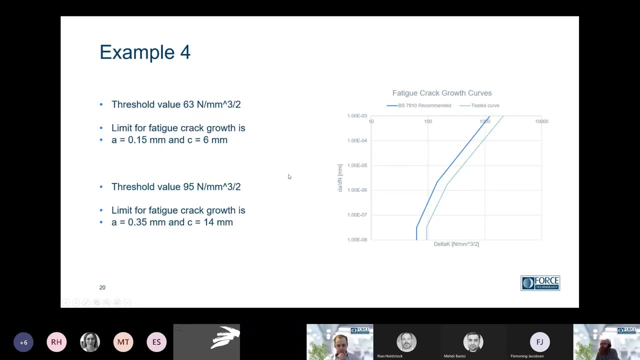 There are a lot of more, A lot more points And the Again The crack grows from the 0.5 millimeters to 8 millimeters. This time it's more than 15 years Before we reach the Critical floor size. 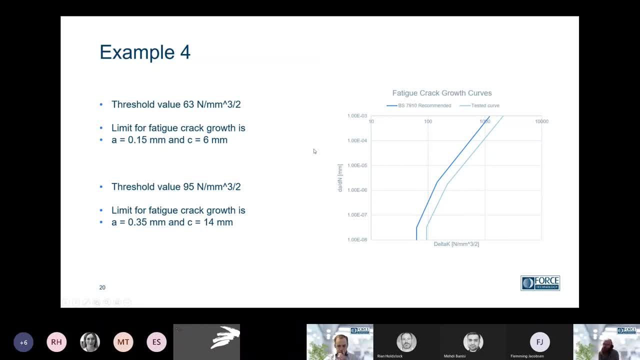 Example 4.. Is the Similar to the two previous ones, But here we are looking at the, The limit for when Fatigue crack growth is actually Observed, And For the BS7910. Recommended curve, The limit for fatigue crack growth is: For a floor size or height of 0.15. Millimeters And the Length of 6 millimeters. If we increase the threshold value By A factor of 1.5. We increase this limit To a Floor height of 0.35 millimeters. 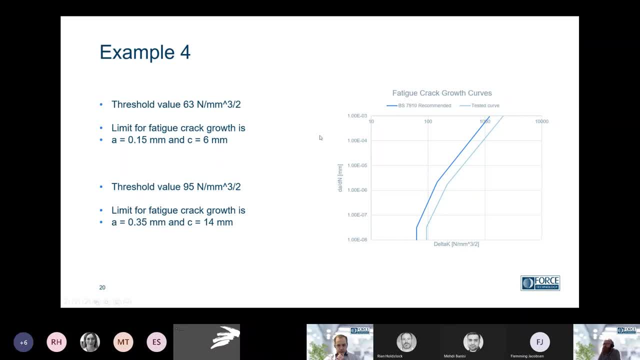 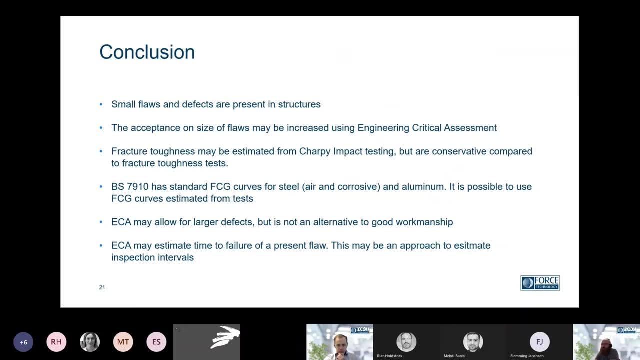 And the length of 14 millimeters. So in conclusion, You can see that small floors and defects Are always present in the structures. The acceptance on the size of floors May be increased by using Engineering critical assessment. The fracture toughness may be estimated from. 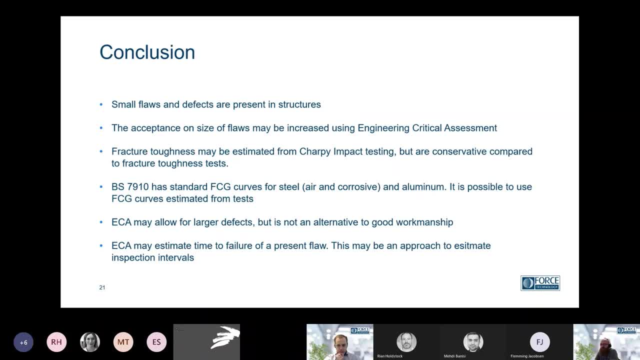 Sharpie impact testing But are conservative compared to Fracture toughness tests, And the BS7910 has standard FCT curves. for steel It's both in air and corrosive environments, And for aluminum It is possible to use. 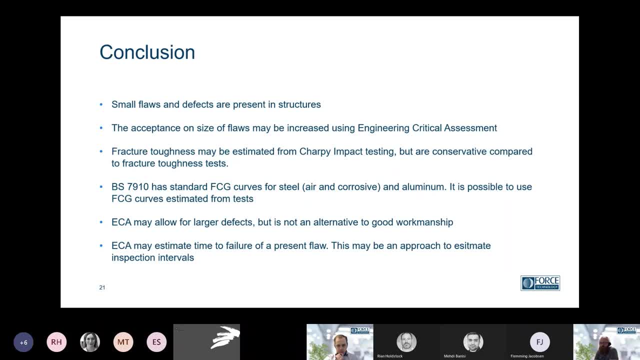 Fatigue crack growth curves estimated from tests. If you have some more exotic materials, You will want to test at specific R ratios And you want to challenge to the Recommended curves in the Standard. As I said earlier, ECA may allow for larger defects. 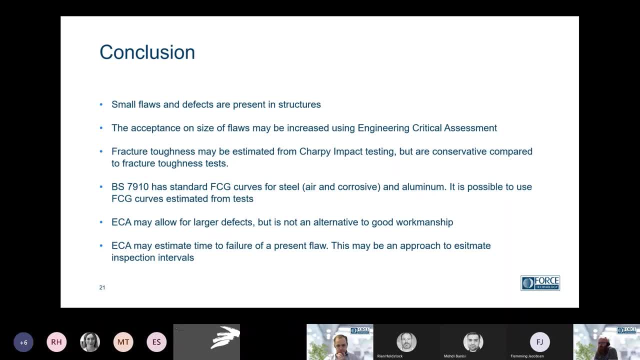 But it's not an alternative to good workmanship. ECA may also estimate time to failure Of a present floor. This may be an approach to Estimate inspection intervals as well. Thank you for listening. I hope you Enjoyed it. 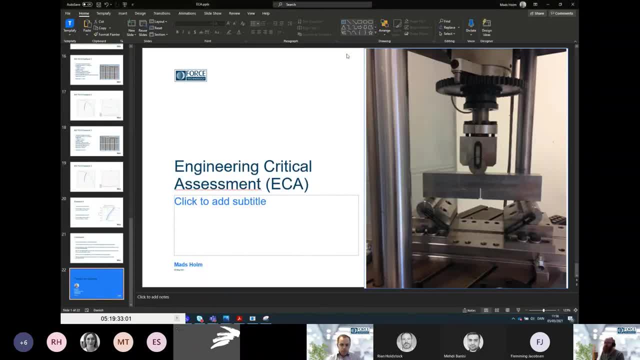 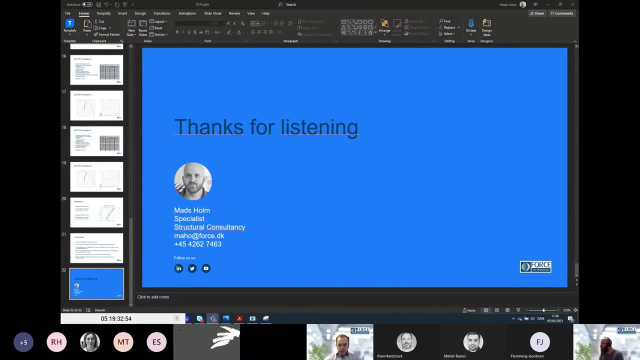 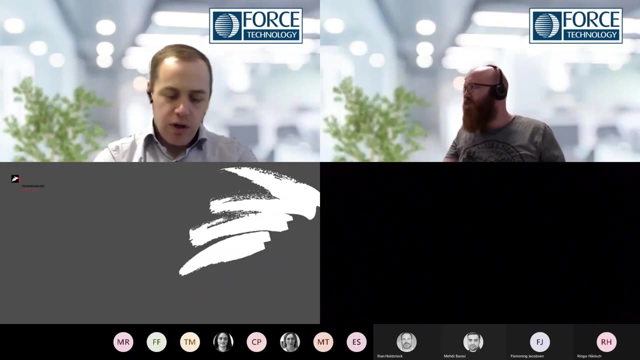 Thanks, Great Mads. Thank you, I think we have time for one or two more questions, If anyone has anything. We also are making a recording of the session And we'll make it available to those that have Attended today. 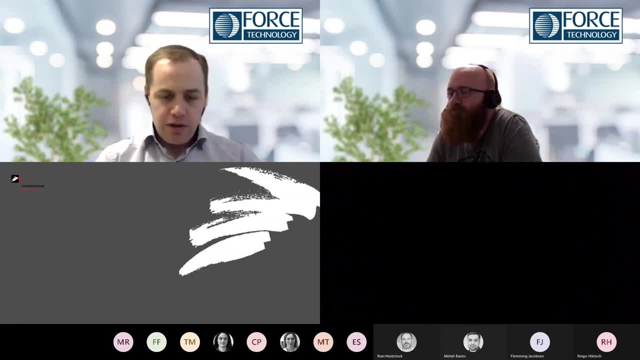 In case they want to, You know, Even just to See the contact details And master me, And if they want to get in touch with any questions later. Does anyone have a question or two Before we have to wrap up? Many. 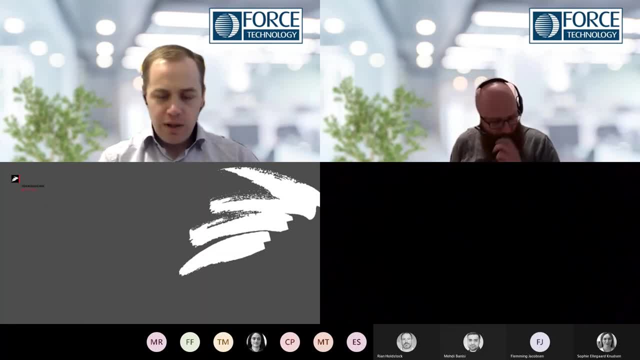 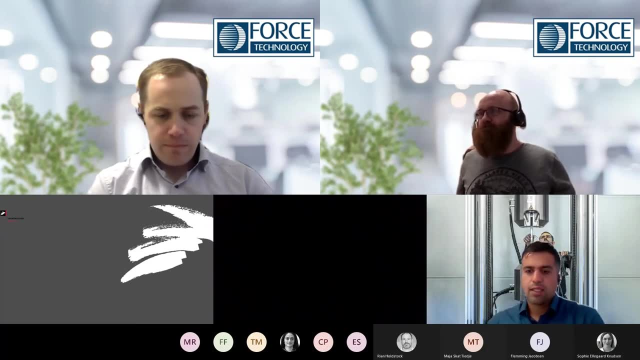 What was the other one you had That you wanted to cover quick? Yeah, Well, there was actually one more for Rhian, But let's take the one for Mads first. There was a question concerning composites, And the question sounds like this: 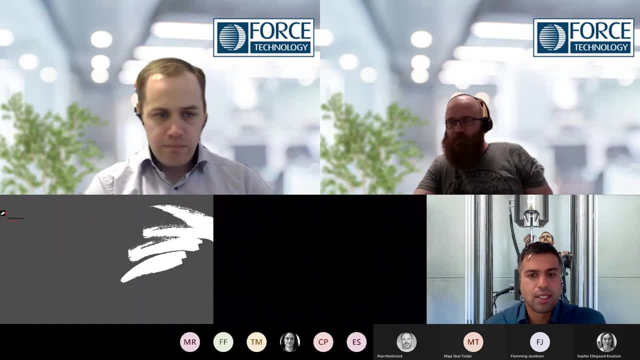 Does the work also apply for composites? I'm not Don't have much experience in composite materials, But I do know that there are some test methods For composites And I've stumbled upon some articles, Also on fracture toughness for composite materials. 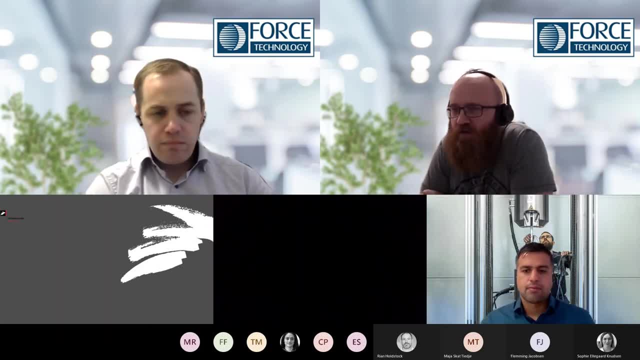 But I must be honest That I do not have any experience with it myself. Okay, But this is basically primarily for metallic materials, What I've been covering. Okay, Perfect, Okay, Okay, Okay, Okay, Okay, Okay Okay. 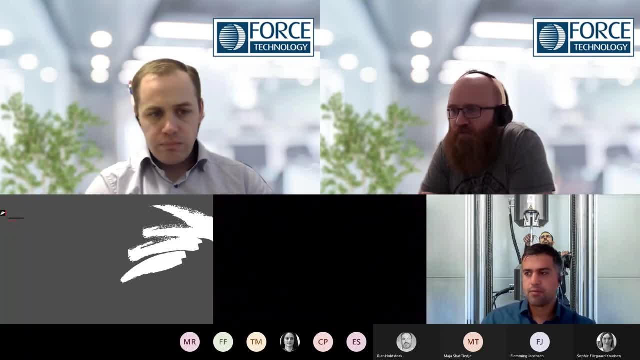 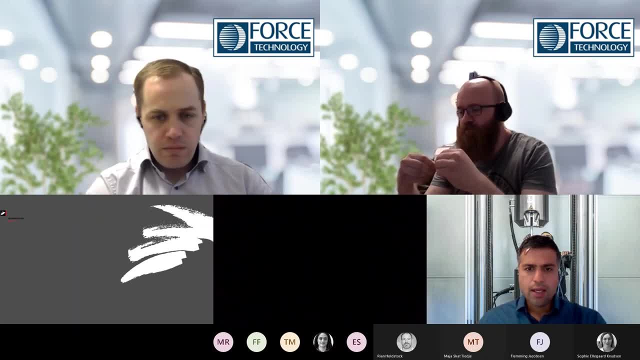 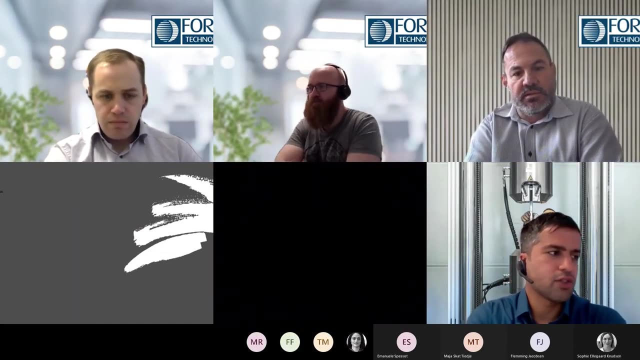 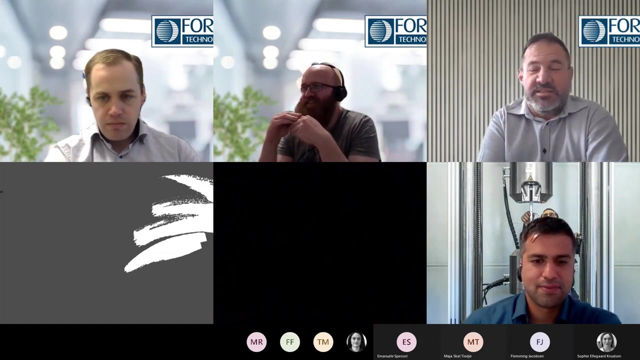 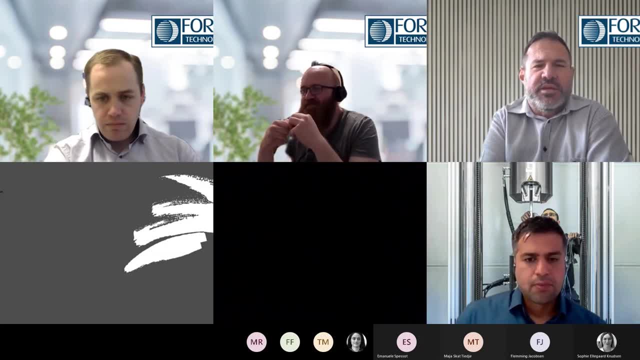 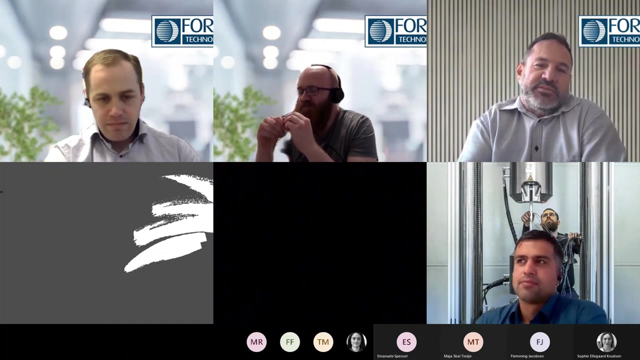 laminate glass and you can give it fracture toughness mass. what's your, what's your take on this? can glass have fracture toughness? I would guess so, but I'm not sure there is a numeric way you know if well it's. I think that's how fractured toughness sort of started by looking at brittle materials, so maybe 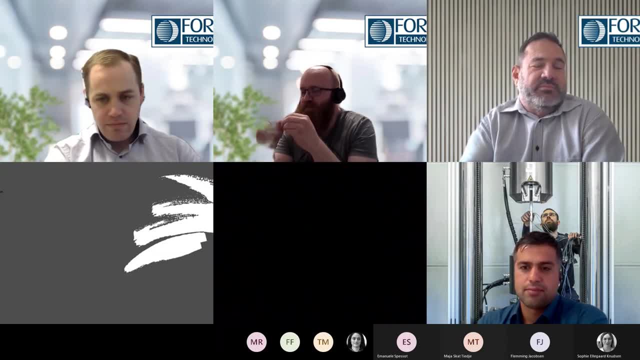 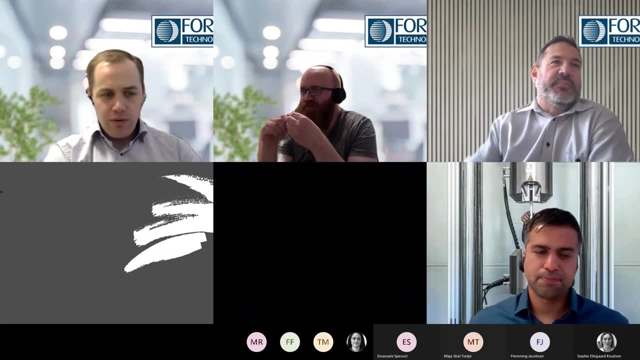 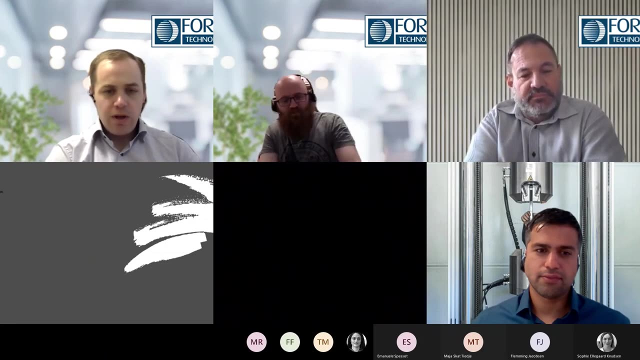 there is something mathematically it can be shown okay, but I think if we get back to the core of, you know, radiance and masses presentations, we were we were looking at an application within metallic materials for those maybe that are working with other materials in other you know that their work. 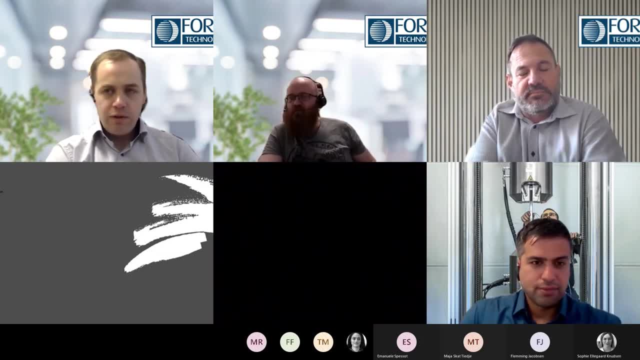 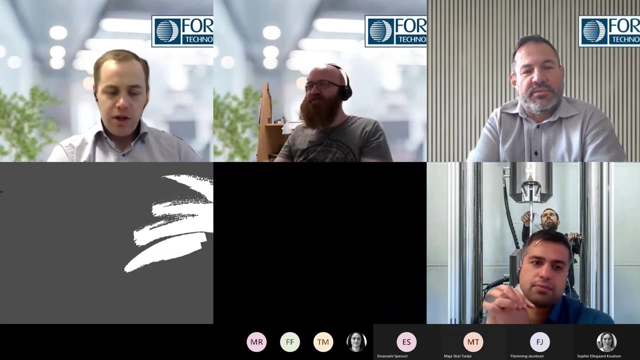 that that in their, in their daily business. we do have specialists also within areas of composites and plastics and glass. I have to check, to be honest. but we have a number of special specialists in other areas as well. where our testing capability is, the physical infrastructure can be used for different sets of materials. so for those that, 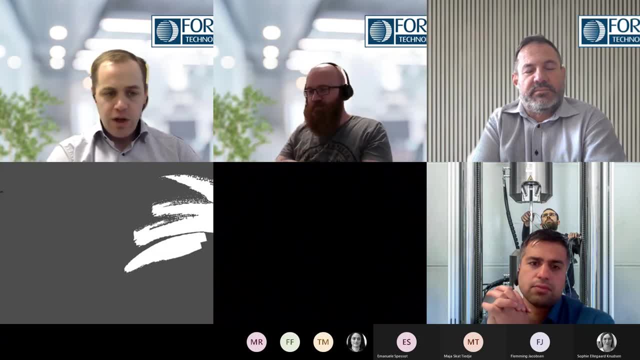 might be interested in working and with different sets of materials and use them on on a daily basis. please feel free to get in touch and we can also connect you with our specialists in those areas. but I do see we're out of time now, so I would like to say thank you very much to everyone that. 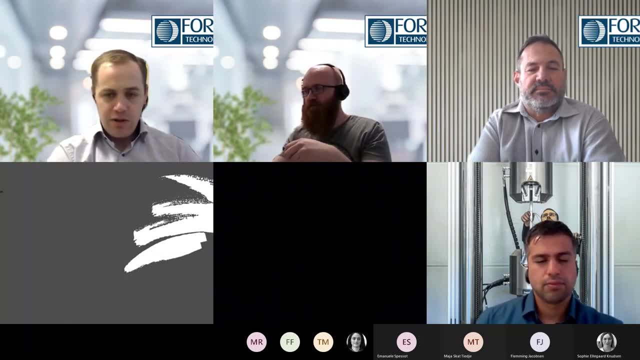 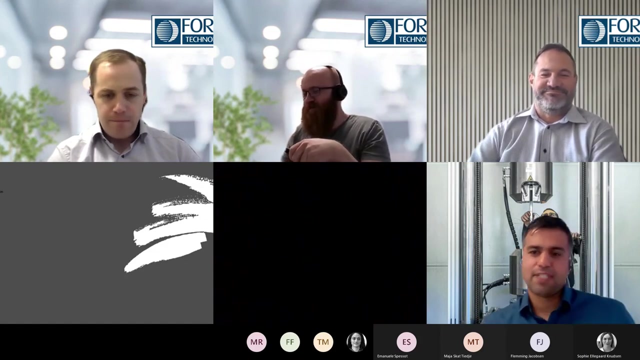 attended, and as well massively, and thank you for the great presentations and if anyone has any questions after the session, please feel free to get in touch with any of us. myself, friend, mass Medi, and we'll make sure we get you an answer to your question. okay, thank you very much and, uh, have a great um afternoon, everyone. bye, thank you, bye.